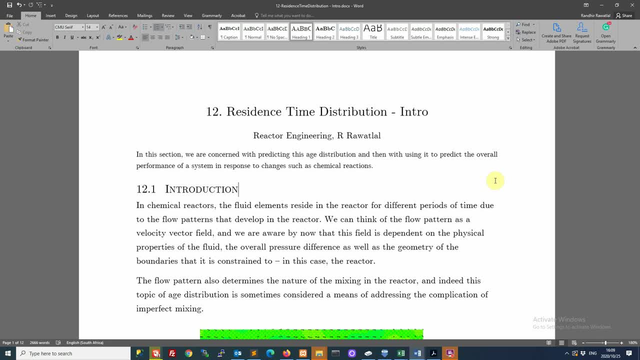 also, we rely on the system being perfectly mixed. In this section we are going to introduce the residence time distribution concept and we'll see how we can use it to examine cases and model reactors that do not exhibit perfect mixing or perfect not mixing behavior. We have been talking about our 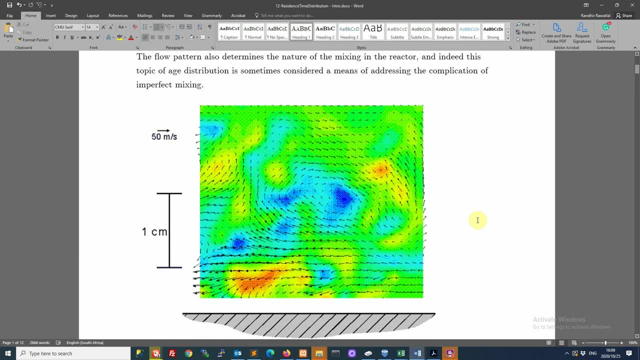 reactor systems in terms of them being perfectly mixed, both in terms of the material and energy distribution. Now let's talk about a more real-world case. So in a real reactor, our flow patterns may be complicated like this. So in this diagram we have the arrows showing us the direction of flow. So our system. 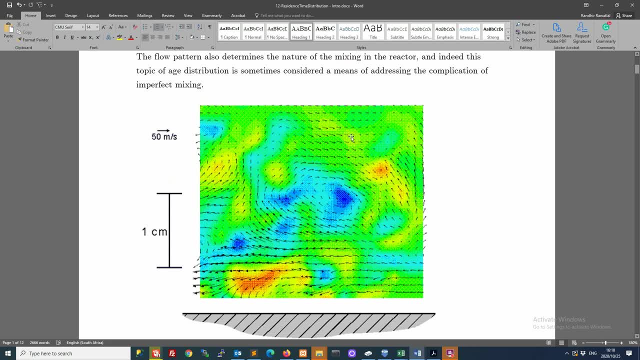 might not be flowing in one direction, or it might not be perfectly mixed, which would show up as turbulence. It might have flow features in it which reveal different types of zones in the reactor, and that's in terms of the flow. That may also be true in terms of the concentration and temperature fields. So 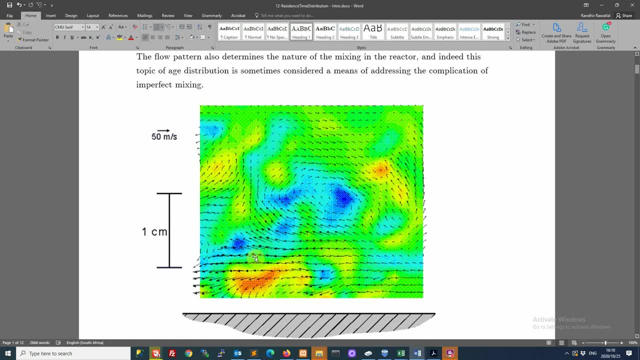 you might have low temperature regions and high temperature regions, or low concentration regions and high concentration regions. So we can imagine, near the inlet point there might be a high concentration of reactant and so on. So in real reactors all these things happen and we then are concerned. 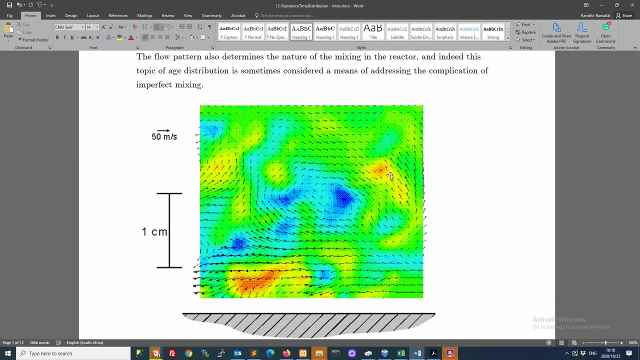 that the models we've been developing no longer apply, that they are based on such restrictive assumptions that they will hardly ever reflect reality accurately, And if that is a concern, that is a serious. that may be a serious issue in terms of our ability to predict what that reactor will do. 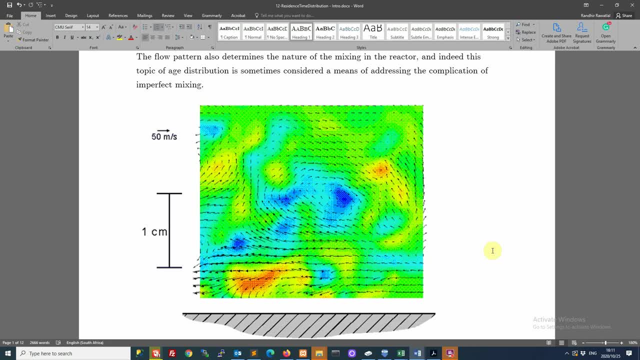 So up to now we've been estimating the reactor volume or developing an energy balance based on the idea that we can estimate a reaction rate for the reactor. So we happily wrote: minus RA equals KC something. Now, if we look at a picture like this, we can see different temperatures, different concentrations. 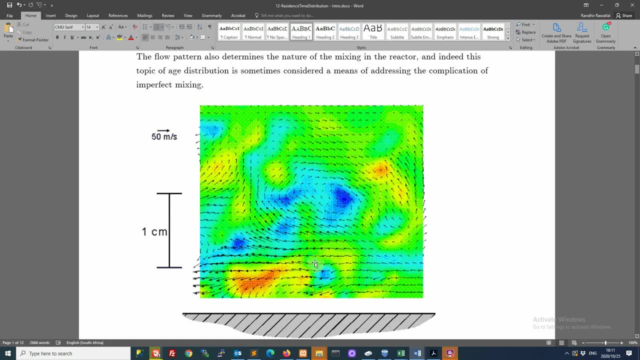 So we will have different reaction rates at different points in this reactor. Also, in terms of the flow, we don't know how to handle the situation where the system is not fully turbulent, and hence perfectly mixed, and it's not flowing in regular straight lines. 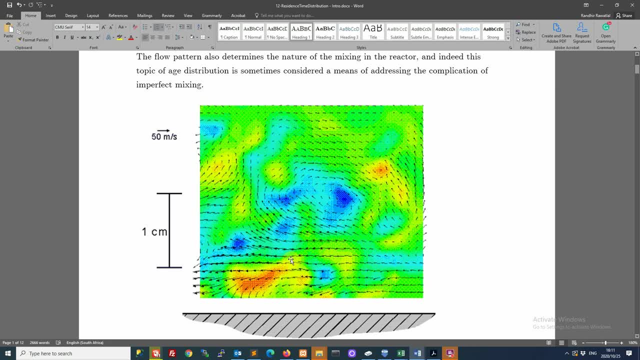 So if we have some other strange types of mixing pattern, Then we are not clear about how we can model this. We don't know how to account for flow into or out of a region And, as we'll show now, the residence time distribution helps us do that quite efficiently. 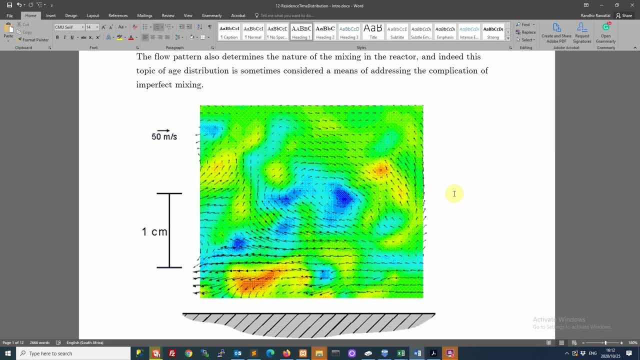 And RTD, as we often call it, is not a new concept. It has been applied very effectively in chemical engineering. But RTD, or residence time distribution, is the same as an energy balance. So it's not a new concept. It has been applied very effectively in chemical engineering. But RTD, or residence time distribution, is the same as an energy balance. 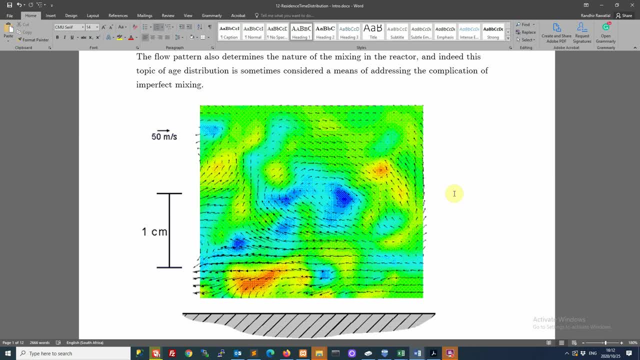 It's the same as an energy balance, It's an age distribution. So when we say residence time, how long has something resided? How long has something resided in a specific space? And in fact we have dealt to some extent with some variables of this nature. 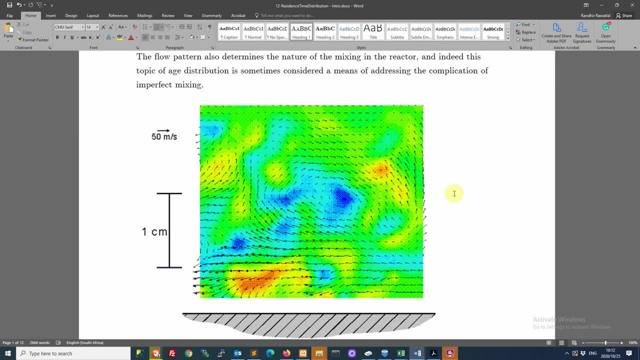 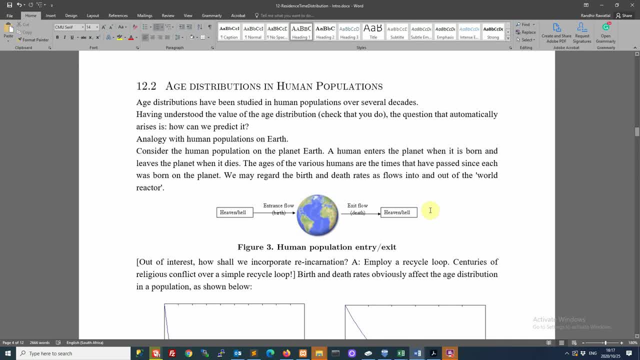 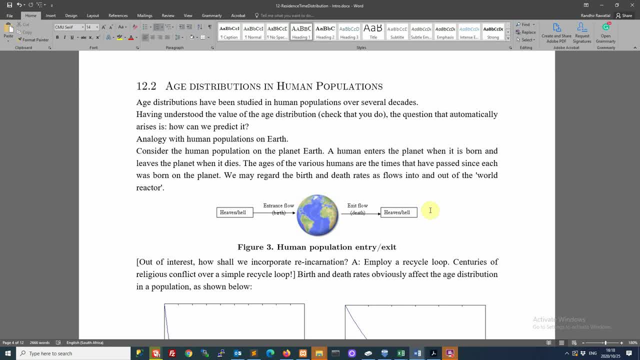 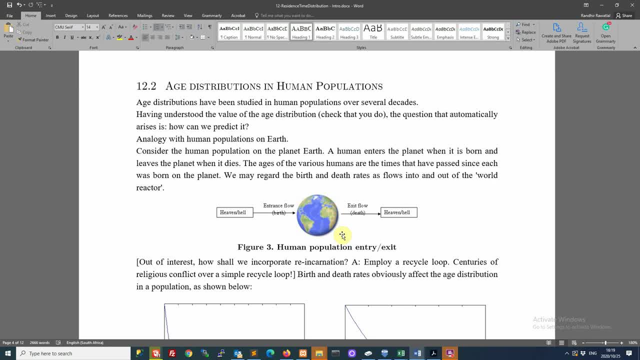 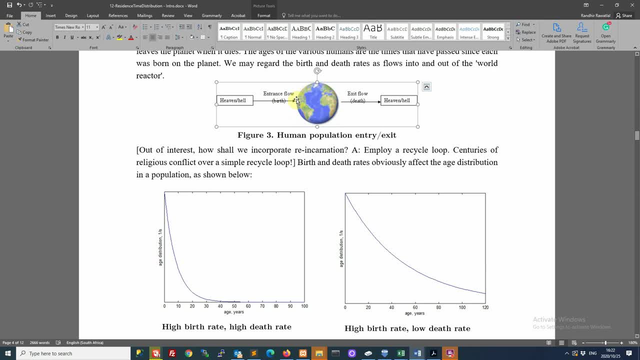 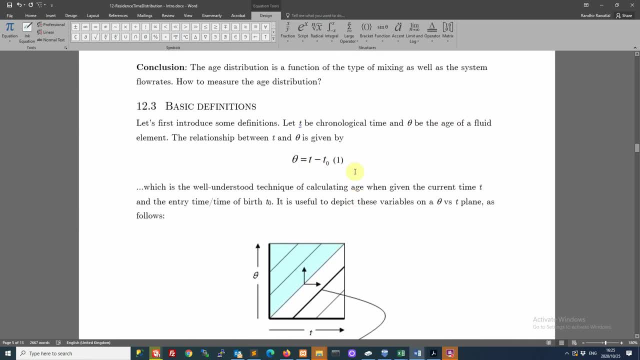 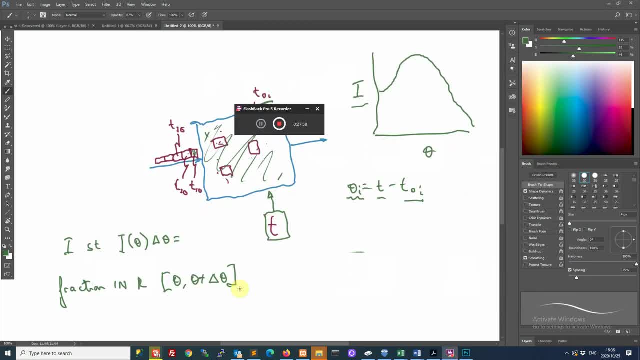 We often talked around the concept that the more time we spent in the reactor, the greater the extent of the reaction. Right so I of theta. delta theta is the fraction in the reactor in the age range, theta two theta plus delta theta, And that's typically how we define any distribution function. 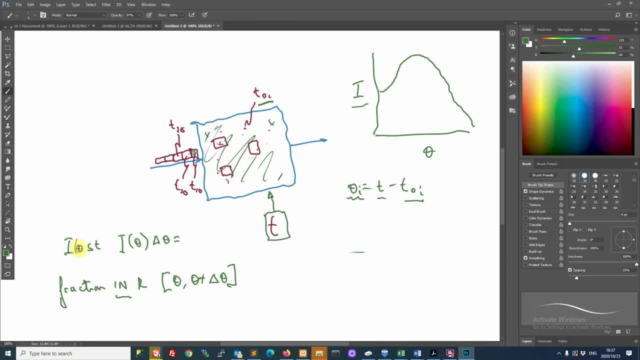 We create a function- right, in this case its I of theta- And we use the function to obtain fractions in specific ranges. And the reason we do it in this kind of roundabout way is because it's very difficult for us to talk about a specific age. 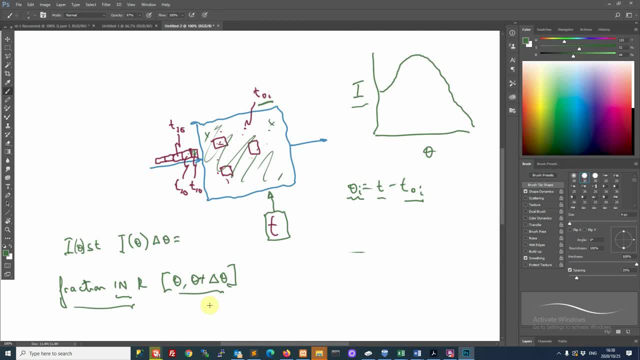 So, for example, if we take a human population, if you ask someone or if you- well, let's say, you ask someone their age and they tell you: I'm 20 years old. Now, there's implied in that an age range right. 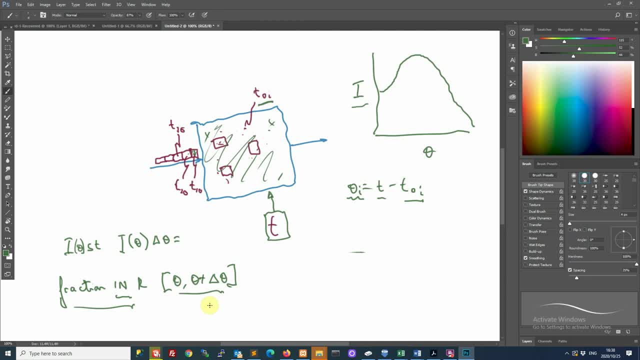 If you say you are 20 years old, you don't mean that in that instant, when you were making that reply, that you were exactly 20 years old, right? Instead, when you say I'm 20 years old, what you typically mean is I'm 20 years old during. 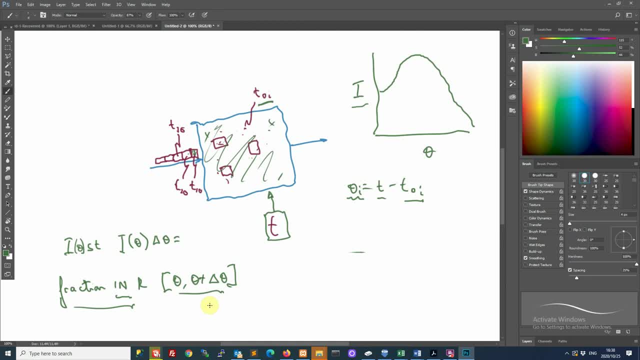 the course of this year, Right Between the start of this year and the end of this year, my birthday fell. my birthday fell within that period. So when you give your age, what you mean is that your age is somewhere in this range. 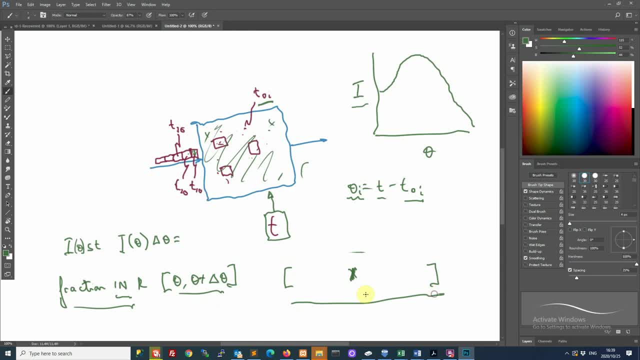 It's somewhere over this span of one year. Now, we do that because it's pointless information. It's pointless information to say I am exactly now 20 years six months and five seconds old, right, And that's because, by the time we said that already, it's not true, right. 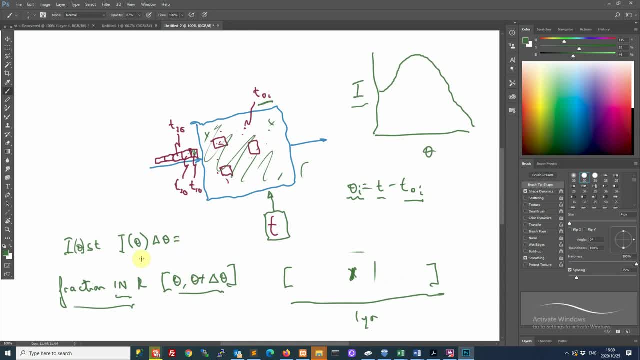 Time has moved on, So we don't want to be so specific about the time. We want to identify fractions over age ranges. Another way to look at it is if we are too specific, Right, If we are too narrow, if we are saying that our age is only in one millionth of a second. 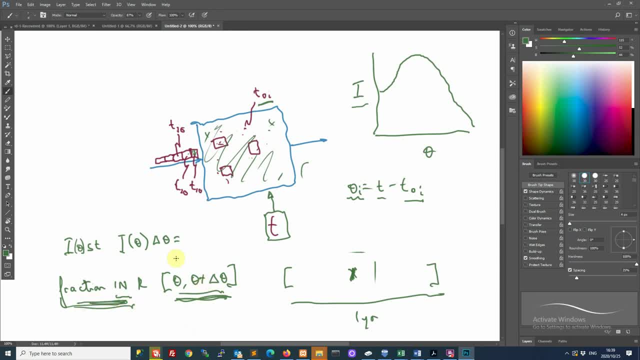 then we will have a very small fraction, right? So that's why we define our distribution functions in terms of ranges. A similar thing with height, right? You can also define a height distribution. So let's say, we want to know what proportion of the population has a height of, say a. 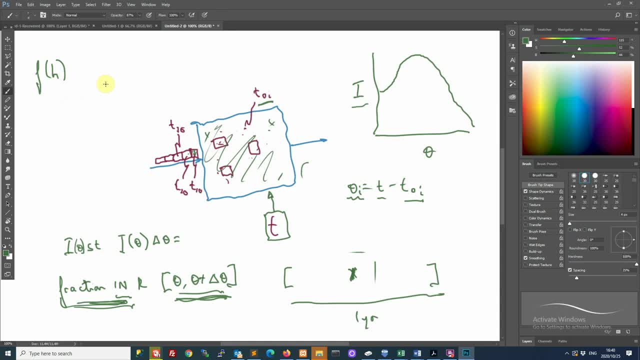 5.5, or let's say 1.7 meters. So when we say 1.7 meters, we typically mean a specific range. We typically mean 1.65 to 1.75,. right, That's what we mean, because there's likely a very small. well, there's likely a zero. 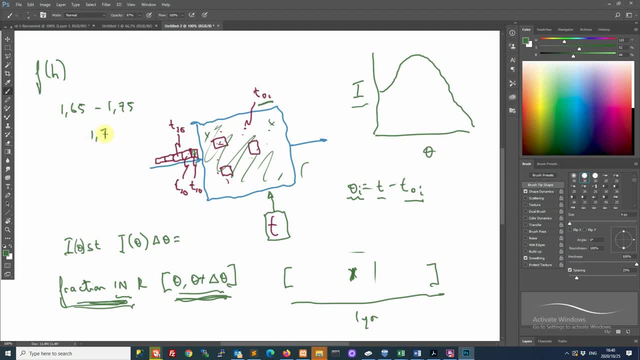 probability that anyone is exactly 1.75.. So that's why we define our distribution functions in terms of ranges And in fact it comes down to how accurately can you measure this anyway? So we have to talk about ranges of things, So we can define a distribution function which purports to be able to report at as small. 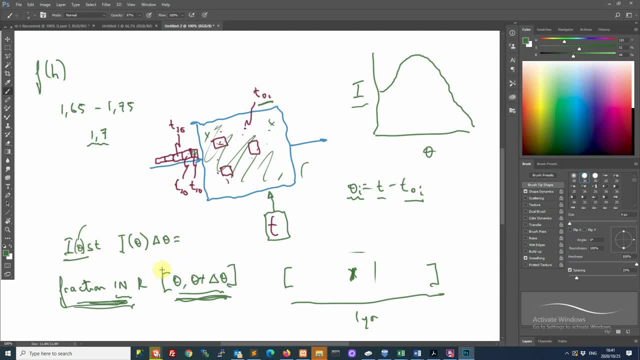 an interval, as we want, but typically from the measurements available, we will be providing data in certain ranges and we will be able to use that to then estimate the function. So anyway, that's the internal age distribution I of theta. That's the age distribution at the inlet point. 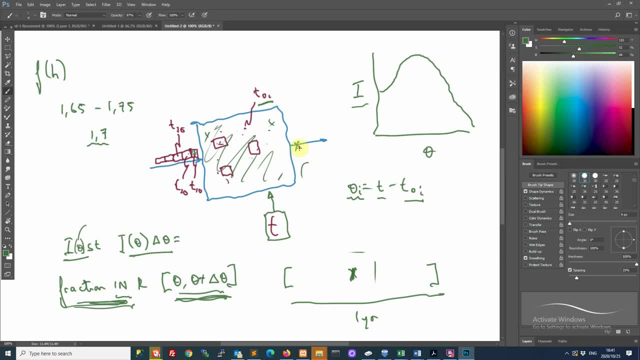 Another age distribution we can introduce is that at the exit point. So we can define at the exit point E of theta And it's the same definition as here, Except that for E it's the distribution at the exit point from the reactor. 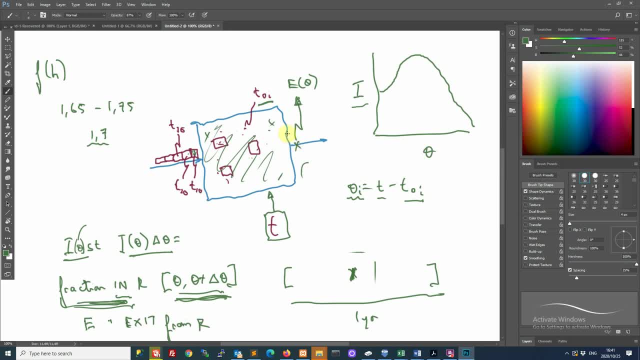 So you could be sitting out here and asking each molecule that comes through: so how long did you spend in here? So what? Only 20 days, That's not much time for reaction. And then the next one comes along. How long did you spend in here? 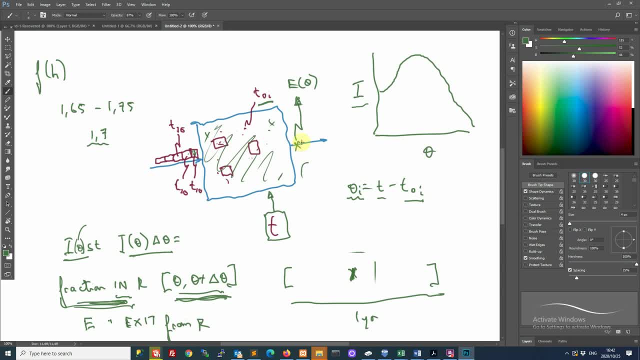 What, only five seconds. You can identify out here the proportion of molecules that have spent specific time ranges in the reactor and are now at the exit point. So E of theta and I of theta, the internal and exit age distributions inside and from the reactor. 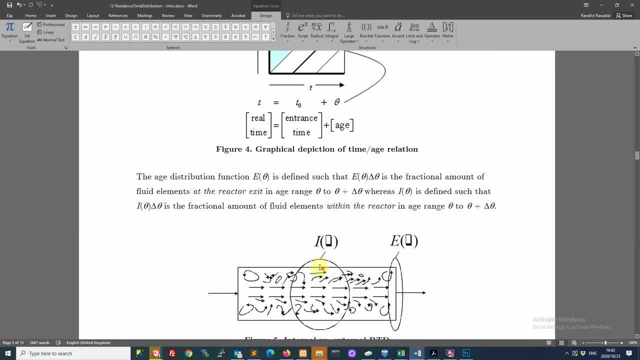 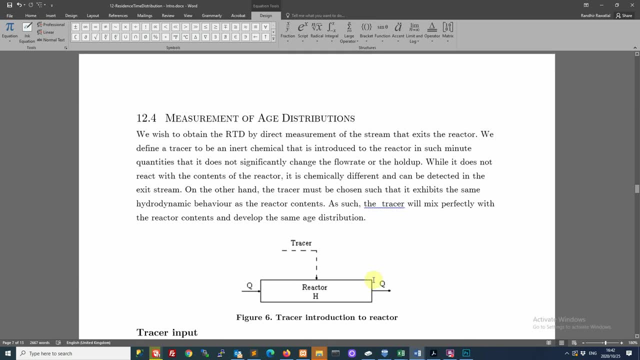 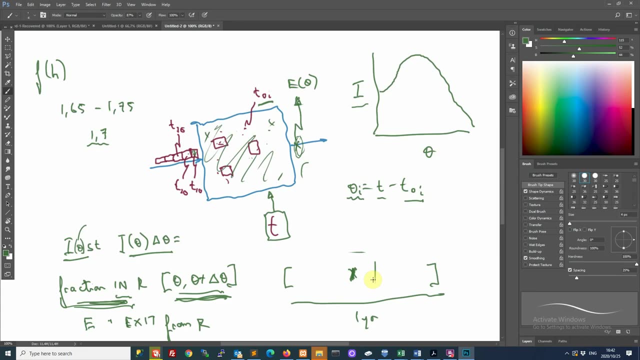 All right. So I and E Now we would like to know how on Earth do we measure these age distributions? If you think about this situation, let's say this was simply water that was flowing through, And if you look at this as a tank here, it's just a tank of water. 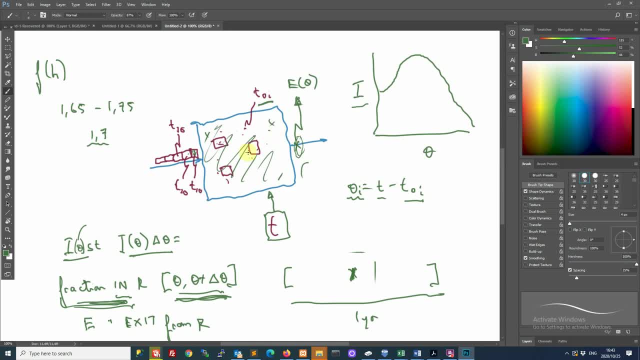 You see no chemical difference between any one molecule and any other molecule. So what? There's just no way to look at the molecules and say, oh, this one has spent so much time in comparison with that one, And that's a little bit at odds with the human populations. 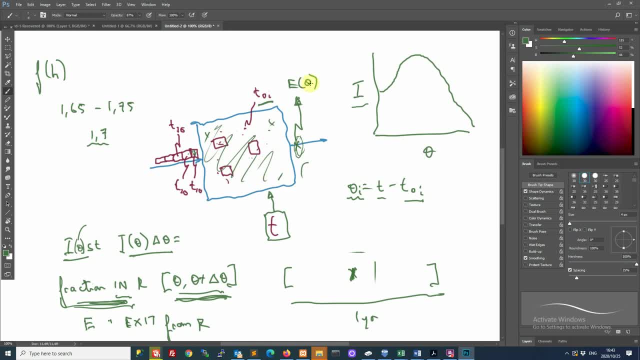 So in a human population you can try and guess someone's age. So if it was a human, if we go back to our world reactor, right, If you were here and you met someone and you looked at them and you said, oh, I guess you are about 35 years old, or something like that. 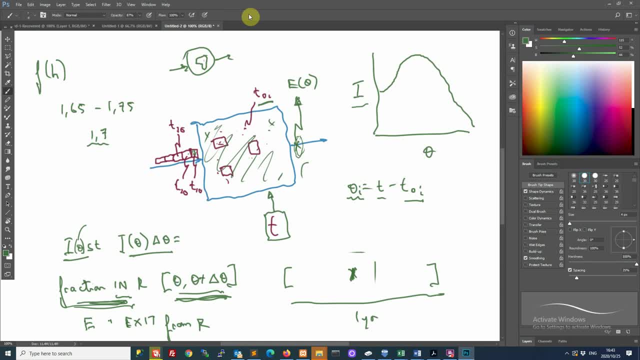 You could do that because implicitly we understand that people, they are born and then they are slowly rotting to death, And so you can observe the signs of that and you can say: well, I estimate you to be about this age, So you can do that with another person. 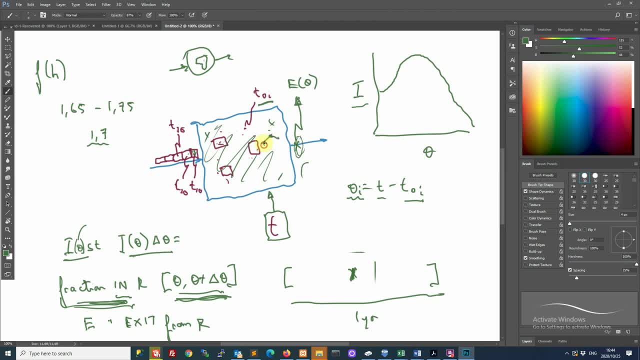 But in something as simple as. Let's assume now we are not looking at decay rates of subatomic particles and so on, that we are just looking at a molecule. There's no observable, there's no way for us to estimate the age of this molecule. 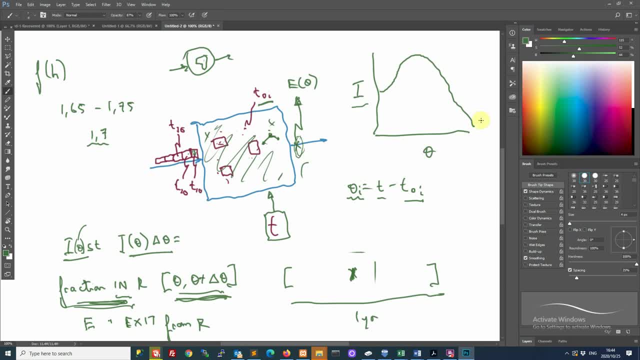 And so we don't try to do that. An alternative is to say: well, what if we put a tag on some of these fluid elements? So let's say, we tagged this, This group of fluid elements, somehow, right? So if we put a tag on all these molecules, then if we observe the molecules here, and then you said, oh, I see. 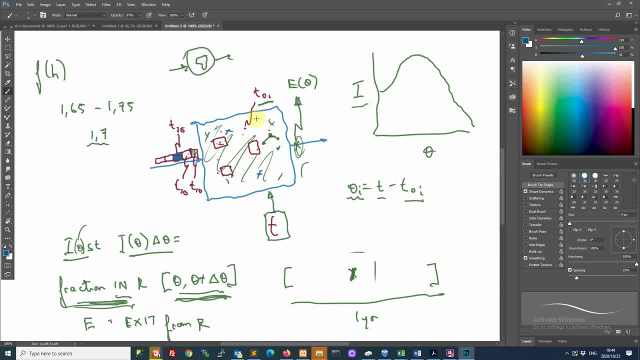 Now we have three of these in this reactor And I know from the molar mass that this amounts to a 2% proportion. So if I know the mass of all the molecules in the reactor and I know the mass of molecules Of this measurable type, then I can say what proportion of the mass in the reactor is of this type. 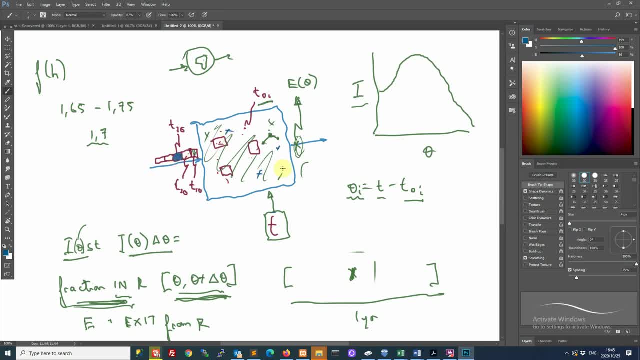 So that's one thing we can do. We can somehow tag the molecules in here, And an easy way to tag molecules is actually not to tag the molecules themselves but to introduce other markers to that same fluid element. And we do it similar to the way I've drawn it here. 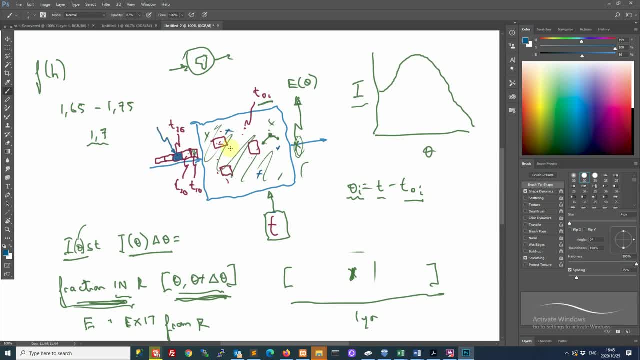 We actually inject something together with that group. So if this is water and if we inject, let's say, a salt solution there, then we know that that salt is mixed with that specific group, And so if we can estimate the proportion of salt that we see in the reactor in comparison with the amount that we put into the reactor, then that's an indication. 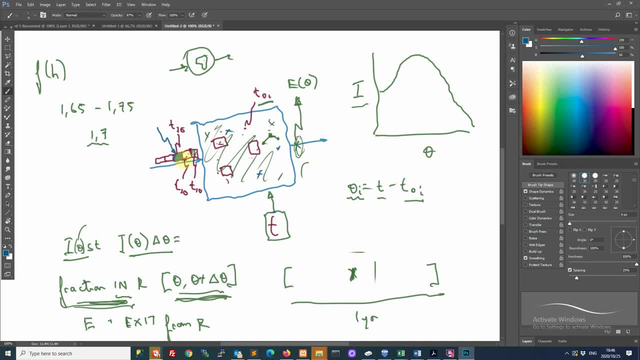 of the fraction that also entered here. So just to say that a little differently: if we know that we've put in originally, Let's say we put in 20 moles of that salt. Let's use a different. So let's say we put in about 20 molecules of salt. 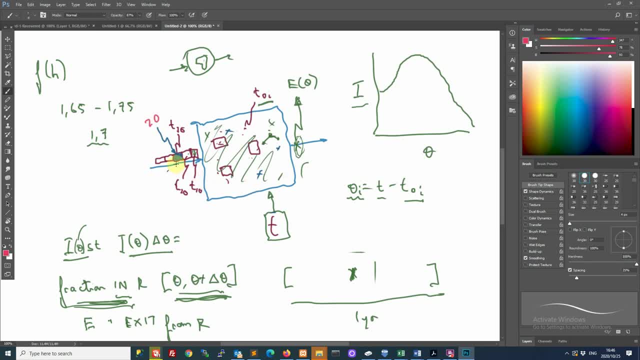 And we did this at some time t naught. So at time t naught we injected 20 molecules of salt in And then, let's say, we looked at the reactor at time t naught, plus 10. So maybe it's 10 hours. 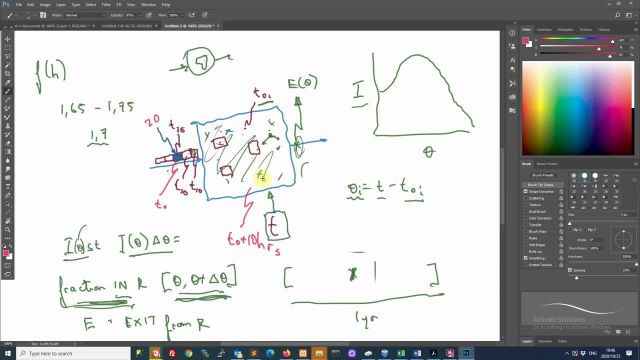 Right. And if we look at that reactor and if we measure the amount of salt in there, somehow we are able to measure it. And let's say we measure that Right. So let's say we measure it and we find that there's just 5 molecules of salt left over. 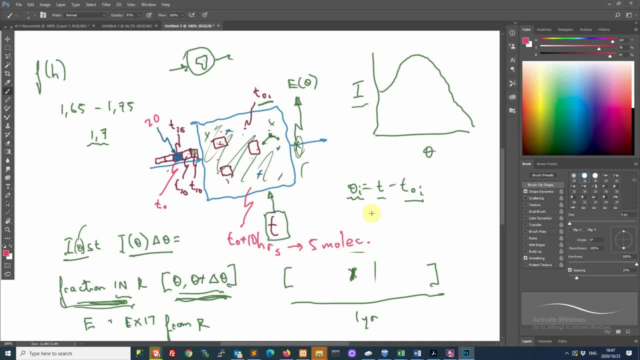 Right. Then we'd be able to say that after 10 hours that our fluid elements will be down to a quarter right, 5 over 20.. So 0.25. And we could do this as many times as we want. 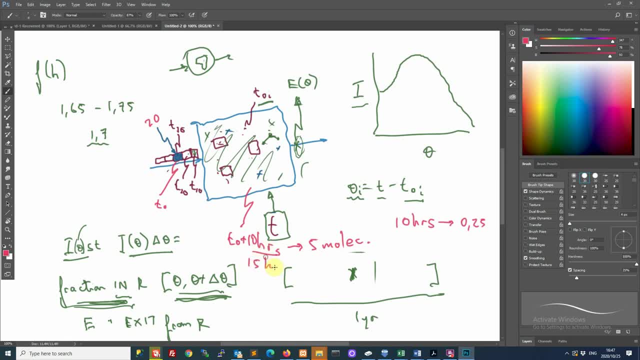 We could ask after 15 hours. So maybe after 15 hours we are down to just 2 molecules, Right? So 15 hours, It's 2 over 20.. So it's 0.1.. And then we could have done it earlier as well. 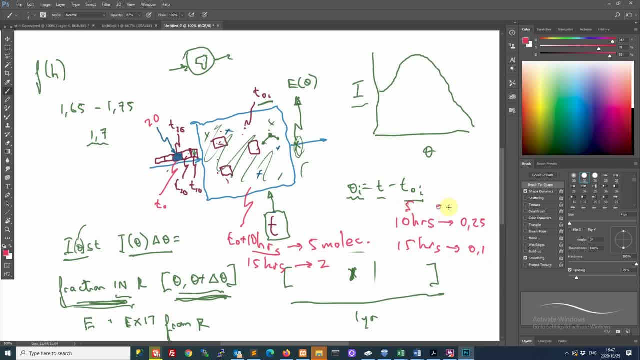 We could have done it at 5 hours, So maybe at 5 hours it was more like 0.7.. And so on. So you see, here This number is then the age Right. We are asking about what happened 10 hours after T0.. 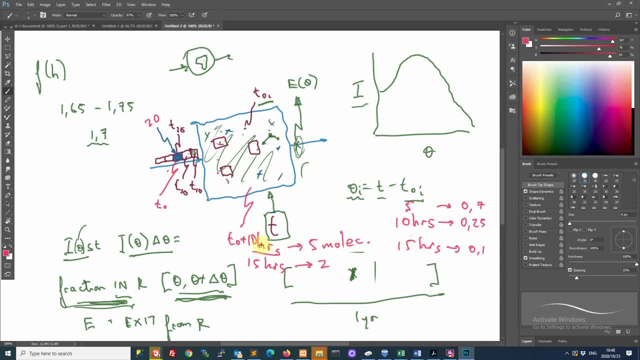 So the age of those salt molecules is 10 hours, And similarly we can ask about the age, or rather we can ask about salt off age: 15 hours, We figure out that there's 10% left, and so on. So in this way we can create for ourselves. 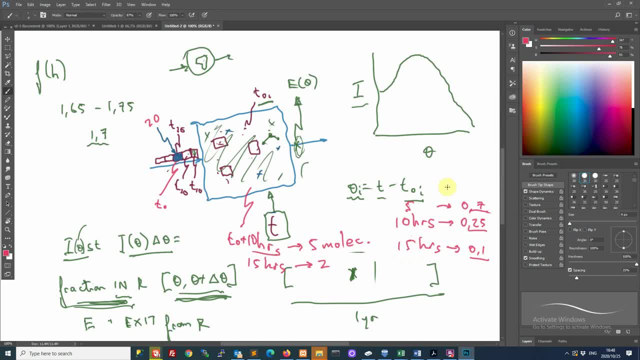 We can create for ourselves a distribution, We can work out what proportion of our fluid elements are surviving to these different ages And we can see. in this case, because of the flow dynamics here, Our salt is running out and after 20 hours there's very little left of it. 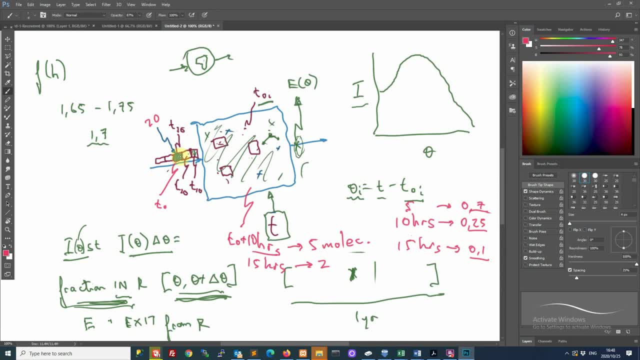 And the assumption that we are applying here is that that salt mixes well enough with the water, That the salt concentrations are a good indication of the water concentrations. So, once more, If that salt is what we call a good tracer, Right If the salt is behaving in the same way. 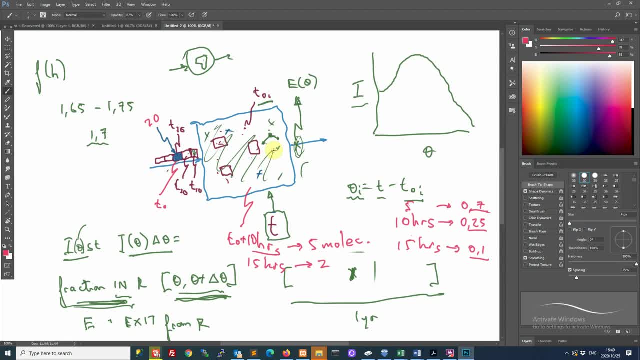 If it has the same flow pattern as the water in here, Then that salt is a good indicator of how the water is distributing itself in the space. So the salt seems to be spending time That looks like this in that reactor, And we are then making the assumption. 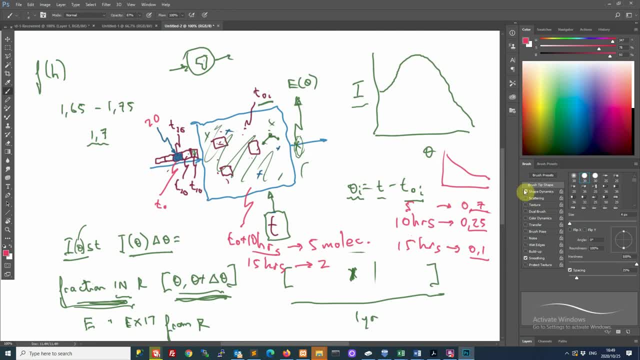 That that salt is an indicator of the proportion of ages of the water in that reactor as well. So that's one way of estimating our age distribution. You introduce something chemically different into your feed stream And then you measure that chemical And from that measurement 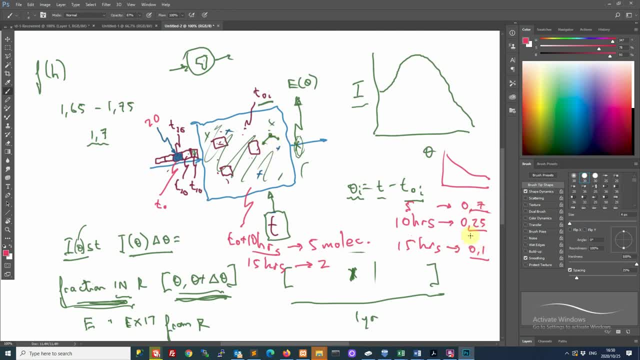 From measurements of this type You construct an age distribution And then you interpret that age distribution of that indicator, Of that tracer, As being identical to the age distribution of the fluid that you are actually interested in- In this case it's the water age distribution. 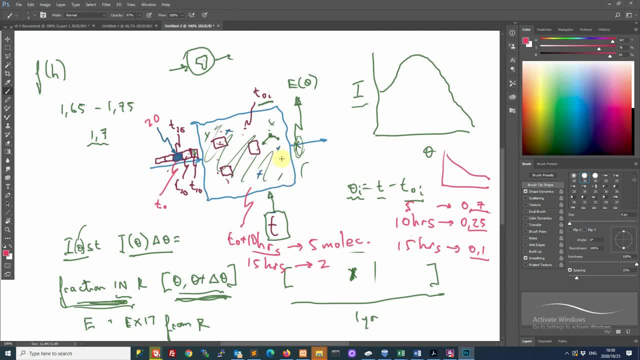 So we can't measure the water directly. Right, There's no chemical difference in the water, But injecting salt is chemically different Because we don't have any other salt in the system. It was only pure water. Now that we have something chemically different, 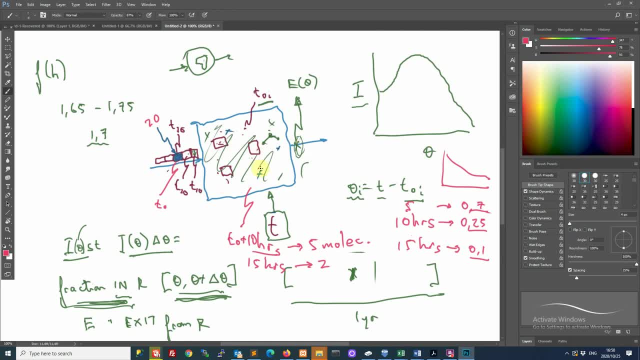 We estimate its age distribution And there from infer the water's age distribution, Right? So here there are little bits where I haven't directly connected these numbers To what does it mean in terms of age distribution and so on? So we'll do all this more precisely now. 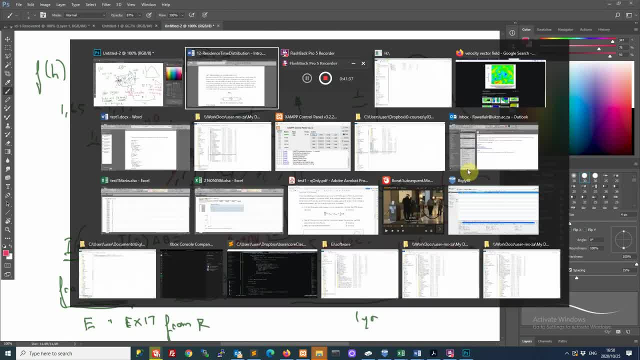 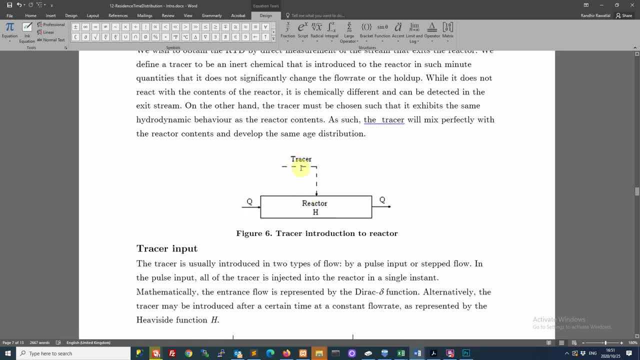 But this is, in broad concept, How we are doing this. Okay, so that's the concept of a tracer. And then again, the tracer must be a good indicator. It must mix well, It must have the same hydrodynamics as our fluid. 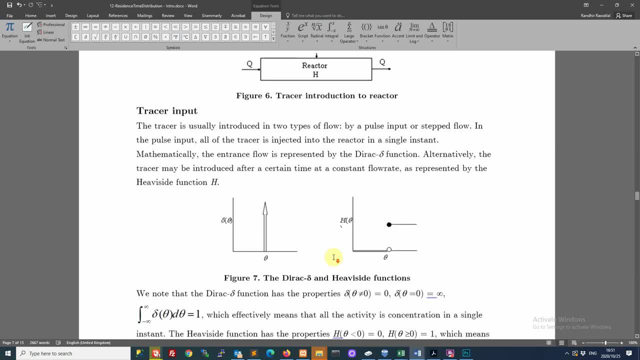 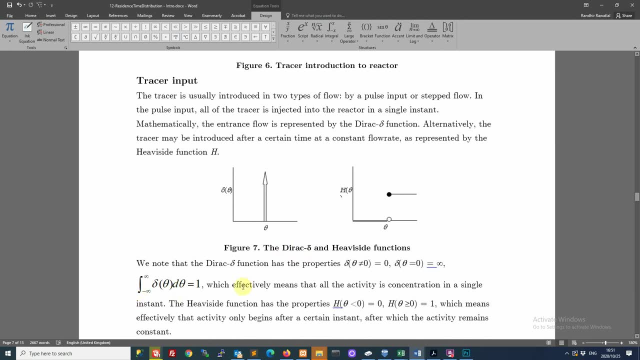 And then we'll be able to estimate the age distributions. And here this is just a comment. We will meet the Dirac delta function in more detail later. So this is just a quick comment That ideally We would just pulse that tracer. 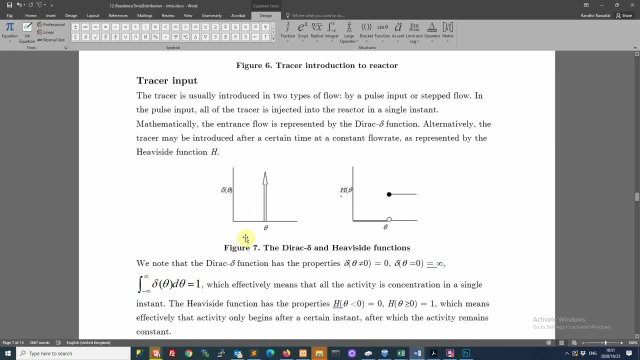 So there are different ways to introduce the tracer. So the one that we just described now was a pulse tracer. So we introduce all the tracer in one quick shot And, in fact, rigorously speaking, Or if you were to represent that mathematically, 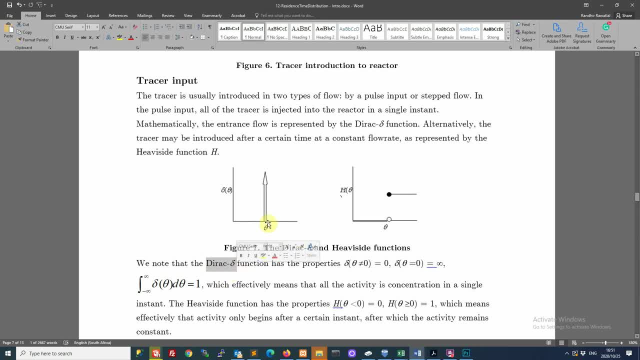 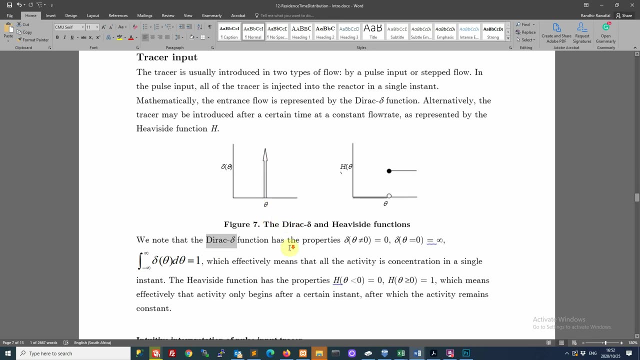 The Dirac delta function is an instantaneous loading of all the salt into that stream And you no longer have salts after that And you didn't have salt before that. So it was just in one instant that you introduced all that salt. So that's the pulse tracer. 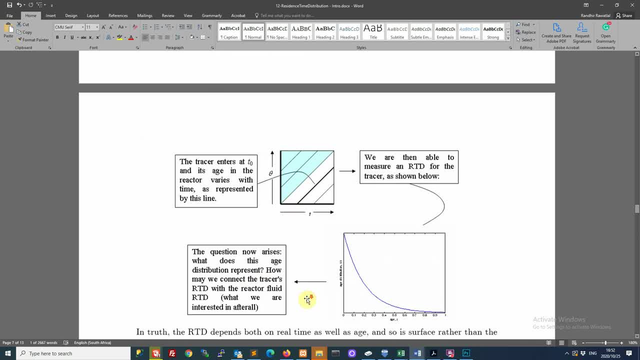 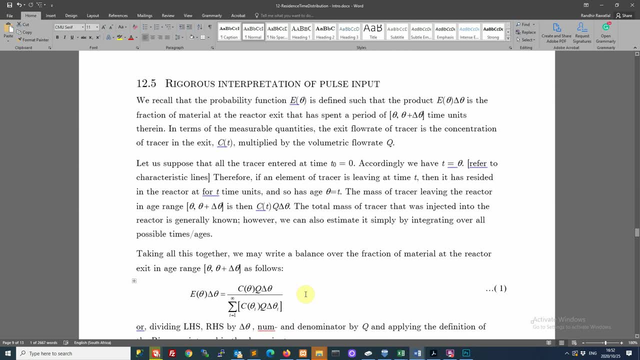 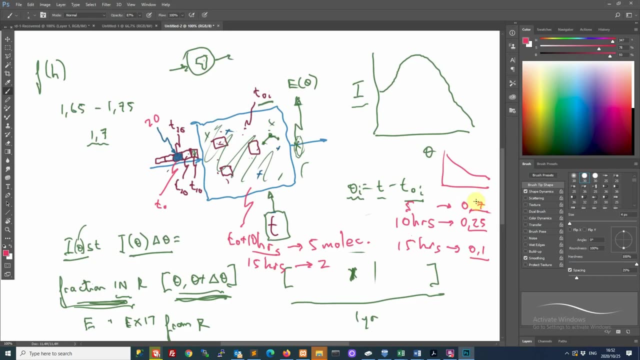 And we'll come back to these diagrams later, But for now, Let's think about writing a mass balance on this. So we have this concept of a tracer, But and we can even imagine, You know, being able to get numbers like this out. 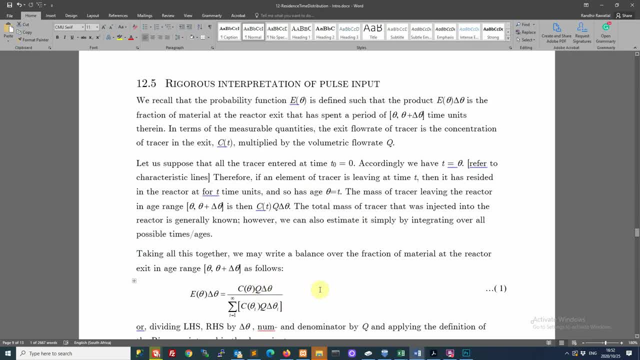 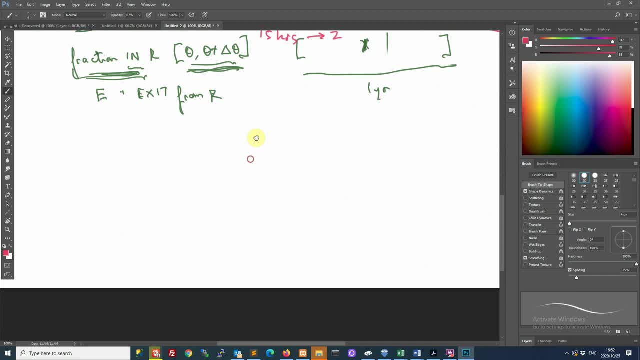 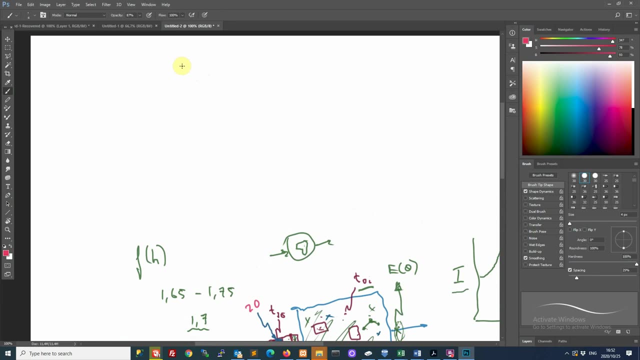 But now let's try to convert that into a distribution function, And the best way to do that, of course, is just to establish for ourselves The mass balance around this. So let's create, Let's say we are doing this in this reactor. 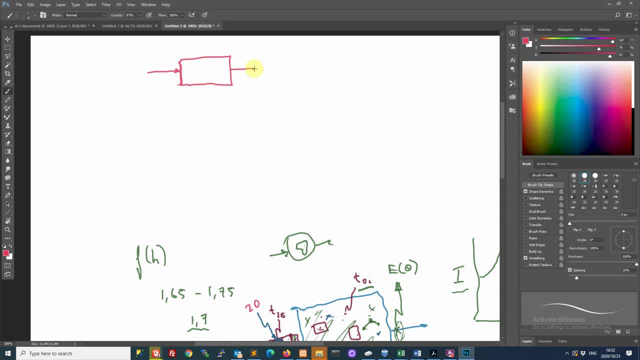 And so we have our flow. So there's some, There's a stream through this reactor, Whose age we are actually interested in, And then we go ahead and we pulse some tracer in At a time that we define to be T naught. 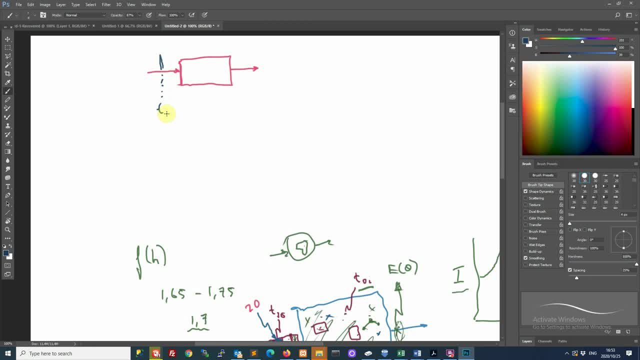 T naught, And so this tracer is going to distribute itself. So after T naught It's going to be distributed in this reactor in some way, And then we are going to start to see tracer appearing At the exit here. And so if you observe at the exit point, 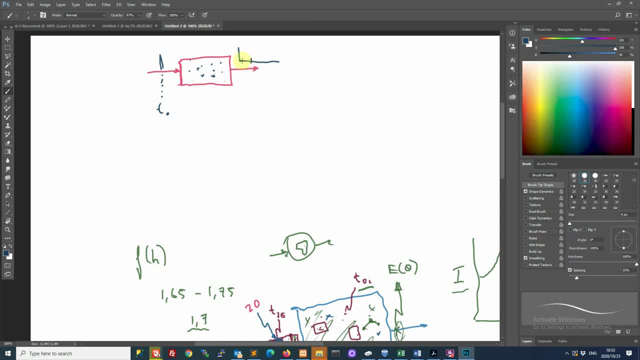 Right. So let's say T naught is here, So at the exit point You will. You won't have seen any tracer, Right, Because tracer only entered at T naught. Then after T naught, You might start seeing tracer appearing at some point. 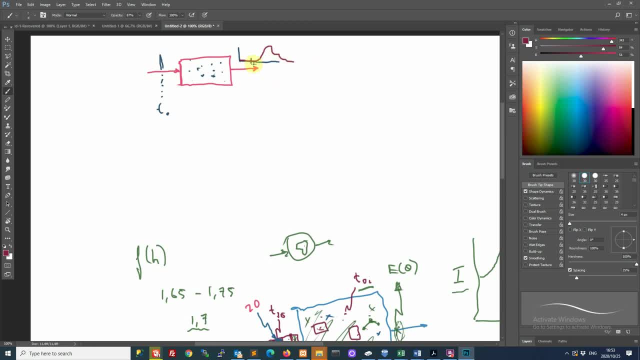 And then You will have washed out of the system. So here We are writing: the concentration of tracer, Concentration of tracer, Tracer, And this is time Right. So here, Now I'm talking about some point at the exit. 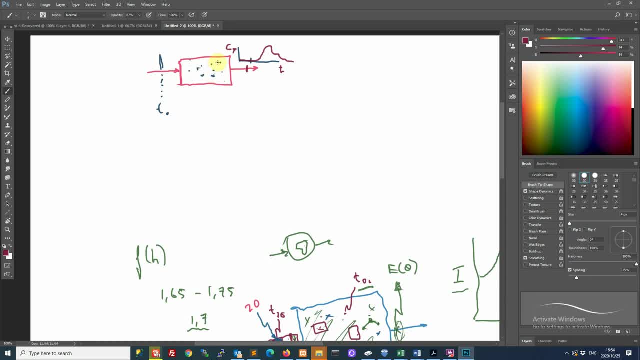 Right. So earlier we talked about measuring the concentration of tracer somehow inside the reactor, And we can't really do that, Right? So, as you can imagine, It's very difficult for us to take samples all over this reactor To estimate the concentration there. 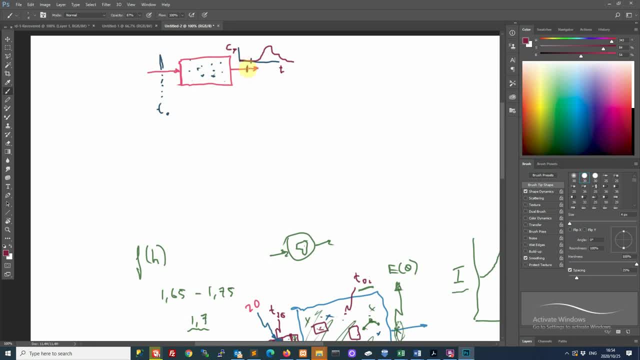 So, more realistically, We can look at the exit point, And we can. We can measure concentration, A salt concentration, As it's varying with time, Right? So we can accept that, Yes, We pulse some tracer in here And then we can observe out here. 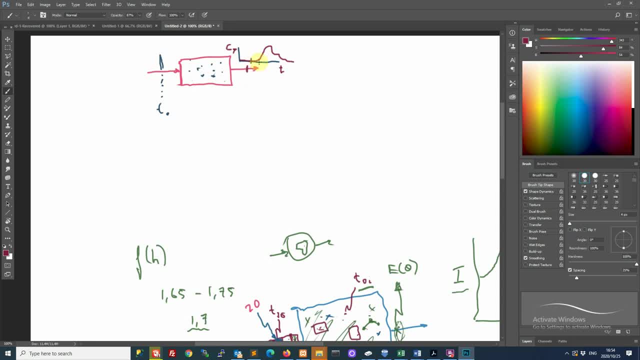 We can keep taking out samples And measuring the concentration of salt In this stream here, So there's nothing wrong with doing that. This is something that's practical and doable in any reactor. Okay, So We have a concentration of tracer. 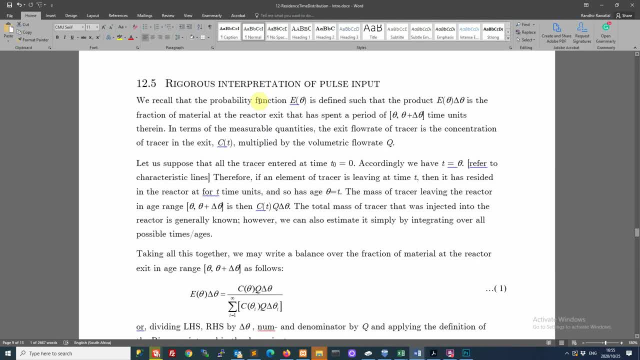 And now Let's think about the mass balance that we can write for that. So first off We can say that Well, There is a certain amount of tracer That That has entered in the first place, But We just think about at the exit point. 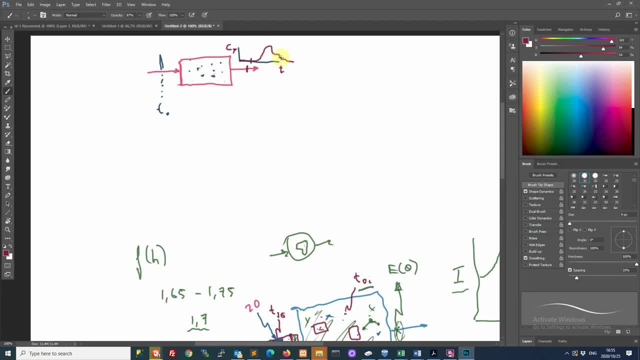 At some time t, Right? So let's pick just some random time t. So there's some time t And let's also pick An interval, Delta theta. So we are going to take some interval here, Delta theta. So 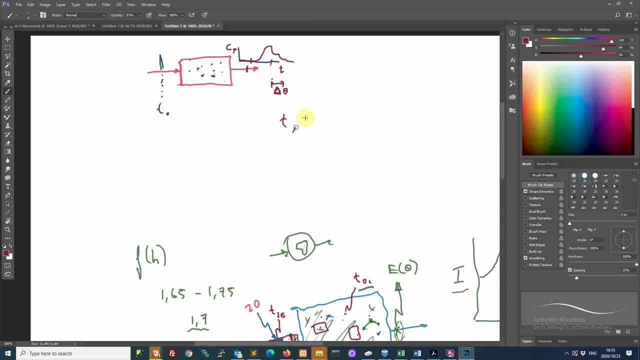 Between t, So between t and t, plus delta, theta. So for example, Let's say t naught was One o'clock, So Thirteen hundred hours, And then let's say our time t, Let's say that was five minutes past one o'clock. 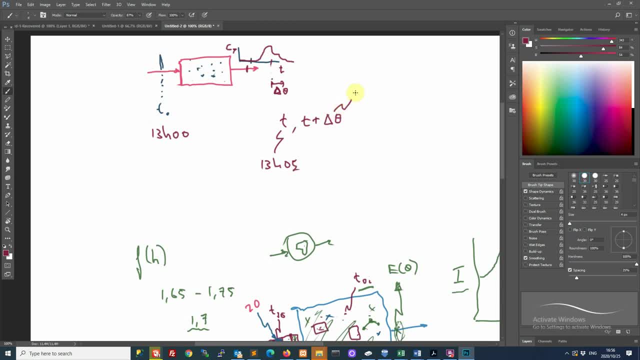 And let's say delta t was twenty seconds. So we are interested In tracer that has exited From that reactor Between Thirteen Oh five And I guess Oh, oh, And Thirteen Oh five, Twenty Right. 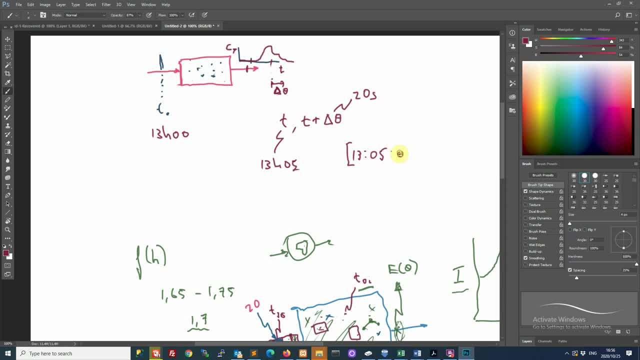 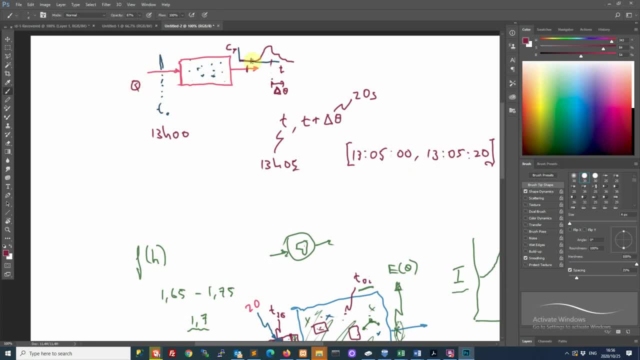 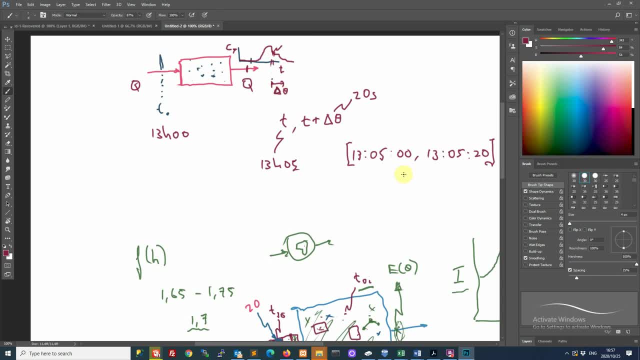 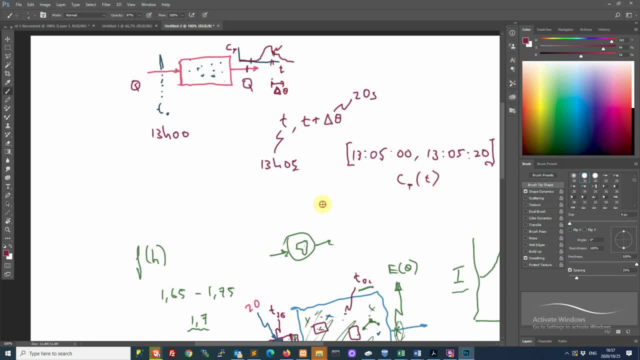 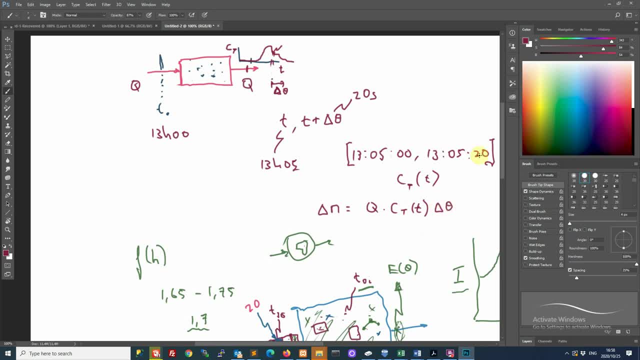 So, So, So, So, So. So here right, delta theta is 20 seconds and our volumetric flow rate is Q and the concentration is CT. so this, if you multiply this together, is the molar flow rate of tracer at time T, and if you multiply that by Delta theta, then that's. 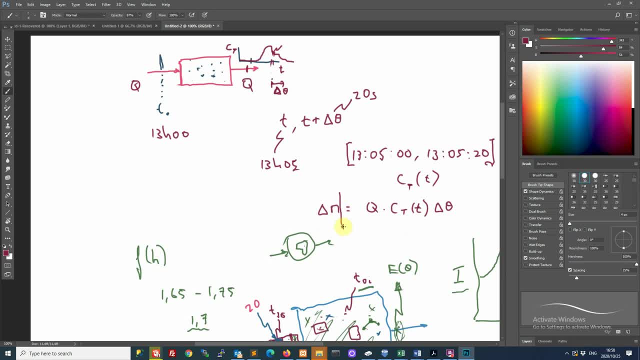 the number of moles of tracer between the times T and T, plus Delta, theta right, that's the amount that left during that time. so that's the contribution from that specific time range. now you you can then say: well, if I go and sit here for an infinite period of time, I will eventually watch all the tracer leaving. 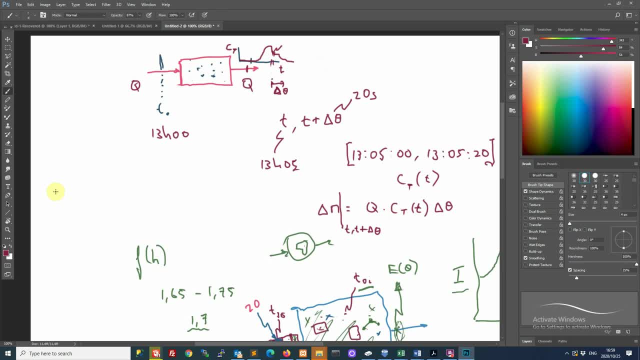 that system right. so you can say the total amount of tracer that I put into the system in the first place. that must equal the sum of the total moles of tracer and what is the total amount of tracer and of all the tracer that comes out here? so the total amount that will eventually. 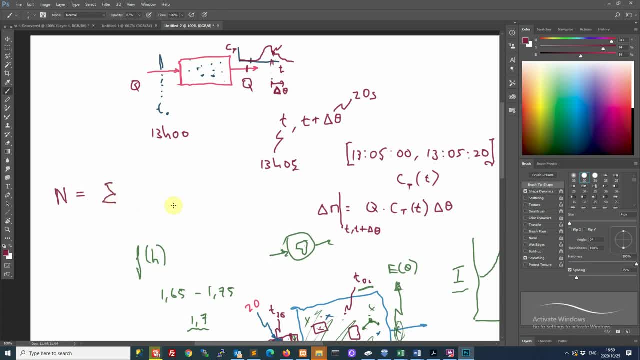 exit is the sum over all those time periods. so Delta, Delta- yeah, I'm just leaving it- Delta in I and that's going to equal the sum of all these things. so it's the sum now. Q, we are assuming is going to be constant, CT, we know is. 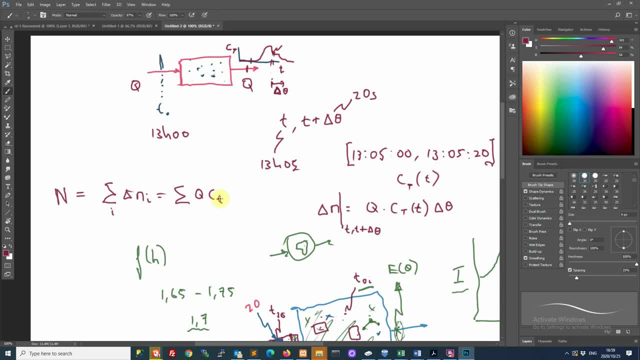 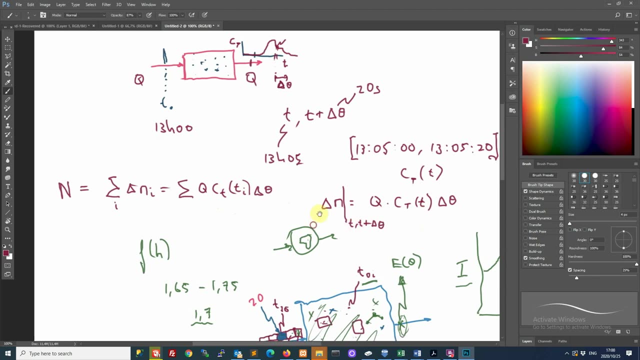 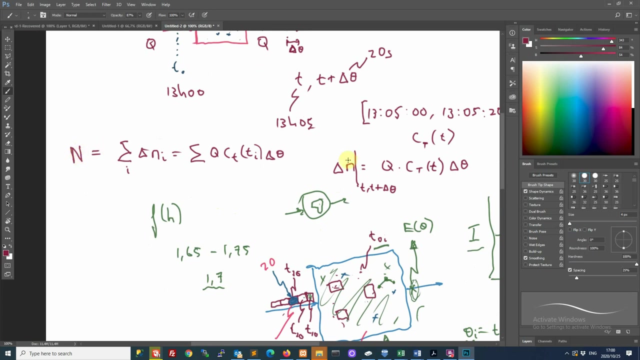 changing CT and this is at TI. so the concentration of tracer for the I interval, and then Delta theta. let's assume we are taking the same Delta theta all the time, right? so this is the total amount of tracer that or that was originally in the system and now this is the amount of tracer that's left over in. 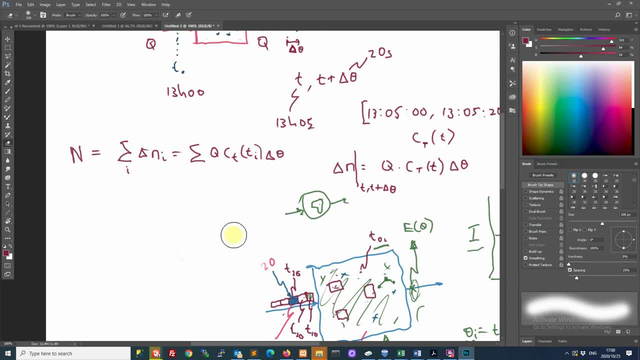 the system. this is clear up here. but if this sum is turned over TW in this, this current is a constant. bring in this over to the two OPAM économique. and then we can say here that the fraction of tracer, so the fraction at the exit between T and T, plus Delta, theta is obviously going to be Delta in over N, and if you compare these two you can see there's a Zar importante summa, a Field, Mozart t, documentение, suite b and IC summa secretary fös, California, c, S, allegro, serie G, GrahamWeamos, Alex, Amick, learn to compute the TapApp, To play around with computers, tape measure. a unitsו� Espada, Theta is obviously going to be Delta in over in. and if you compare these two you can see there's a common Q here, right Q is a constant of Planet Aí and FàngOM월. 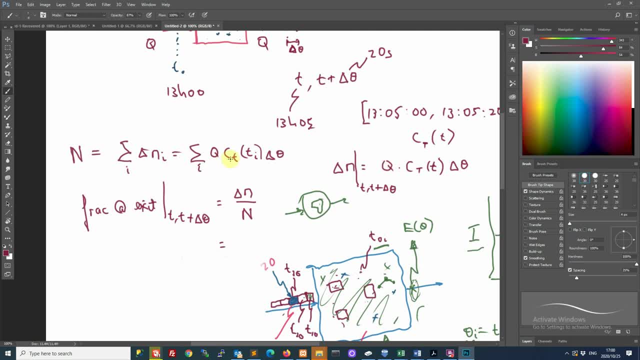 So there's a common Q, which can cancel, and there's a common delta theta as well. All right, and so you're going to get here Ct, Ct, at Ti, over summation, Ct, Ti, And I'm just going to leave the delta theta in here, right? 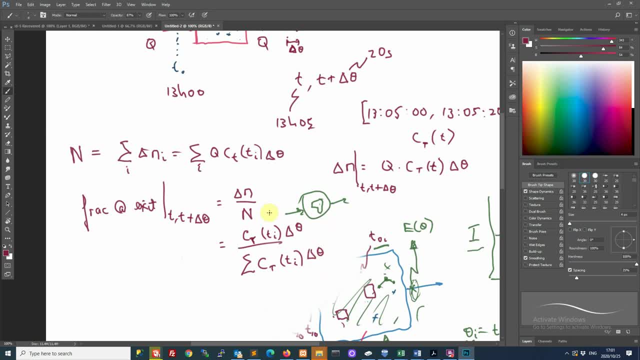 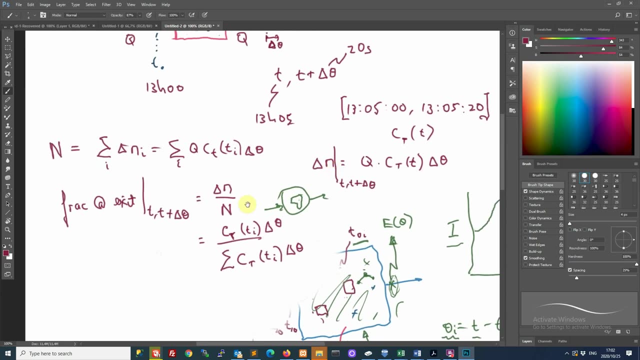 Let's not cancel the delta, Delta, theta, Okay. so the only thing we canceled here eventually was that Q. okay, which is fine. So we agree, that's the fraction at the exit point in this range. So now, instead of a number of moles, we have a fraction of our tracer that exited. 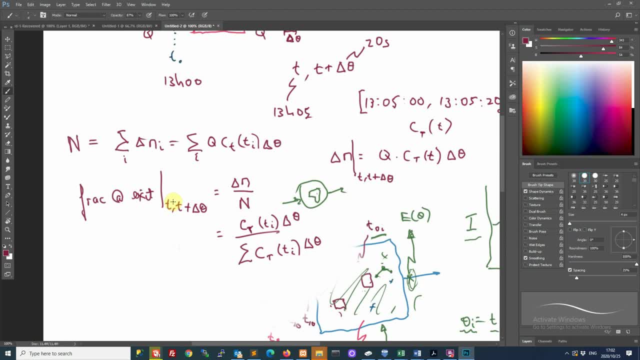 Now, if we think about this fraction at the exit right, remember we had defined the fraction, We had defined the function E of theta, such that E of theta, delta theta, is the fraction of the fluid in that age range. right, So go back and just check you agree. 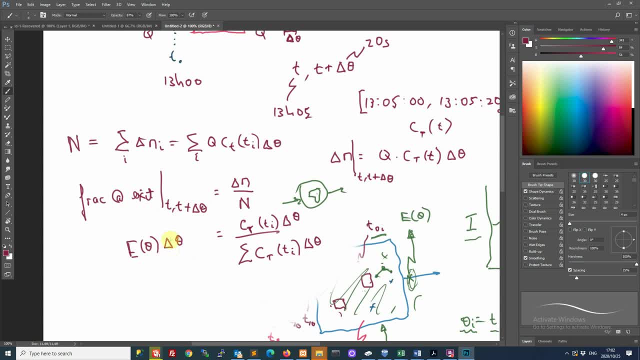 E of theta. delta theta is the fraction, So that was our definition of the distribution function. So that's fine. Now we can cancel this way. Okay, Okay, Okay, Okay, Okay. So let's cancel this delta theta with this delta theta. 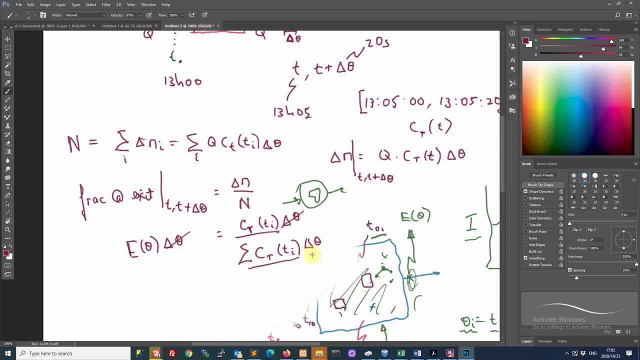 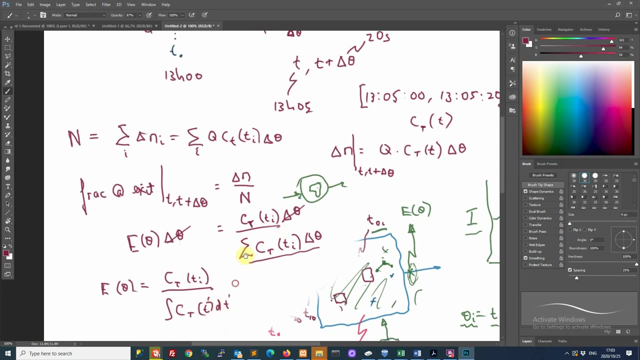 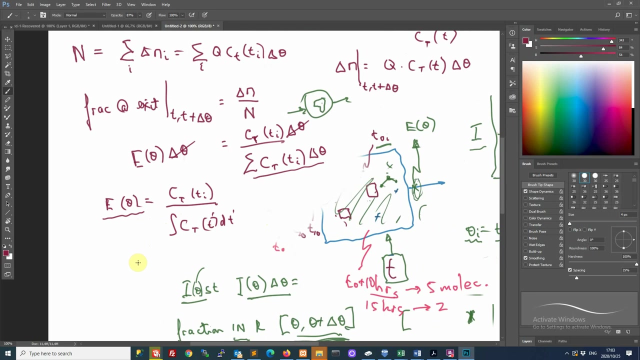 And if you look at the denominator here, you can identify this is nothing but a Riemann integral. In other words you can write here: E of theta is equal to Ct Ti over the integral of E of theta. Then E of theta times this capitalist trial. 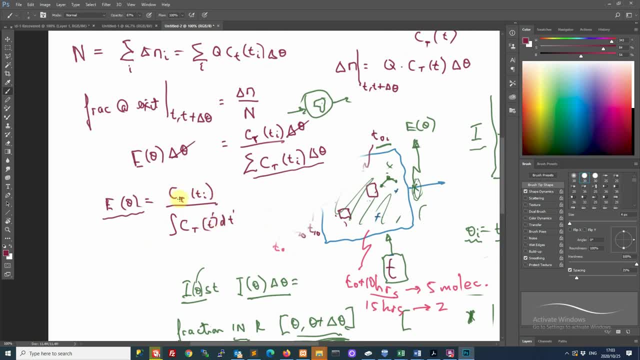 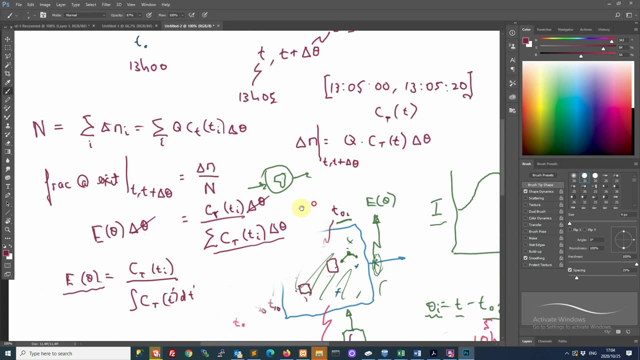 we realise that its anizzy scale. If we want to know the exit age distribution from that reactor, all we need to do is pulse in. some tracers divide that concentration by the area under that concentration profile. so if we think about mathematically what this is right. so we've been measuring the 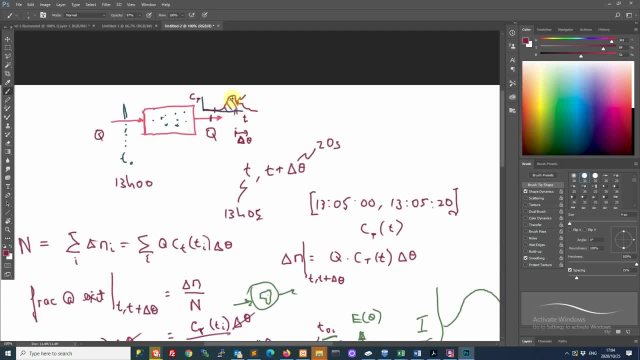 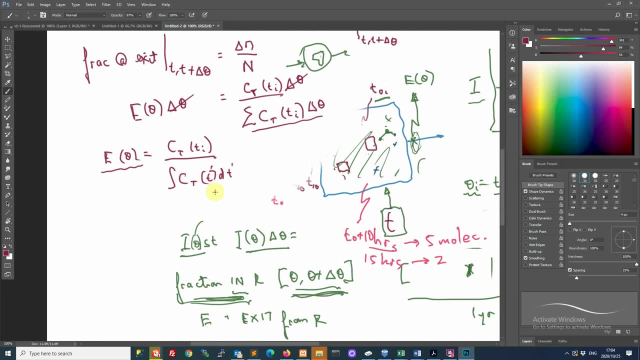 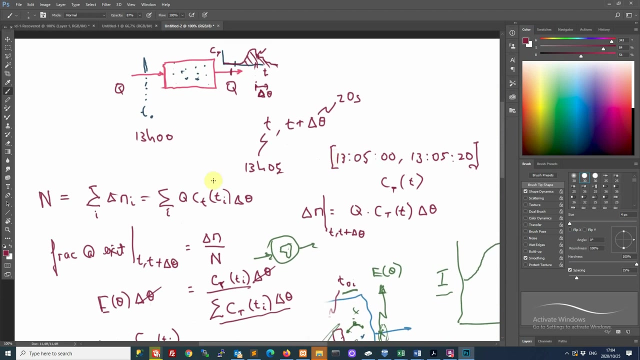 concentration of tracer here, then of course we can measure an area under this concentration curve, and so that's some fixed number, right? maybe we get 10 here, right? and then we just take the whole function, the measured function, CT, and divided by that integral, and that is e of theta. so that is all we need to do if 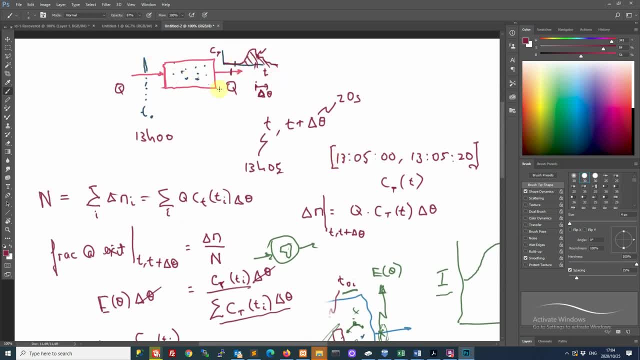 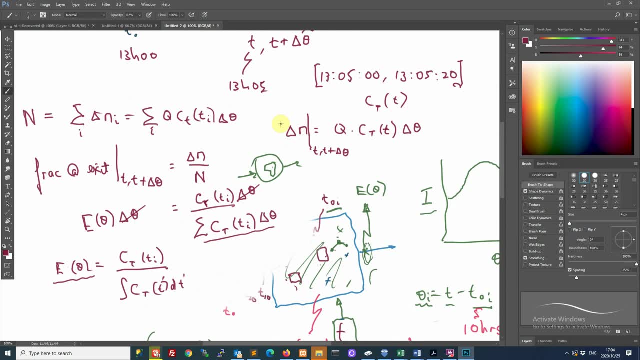 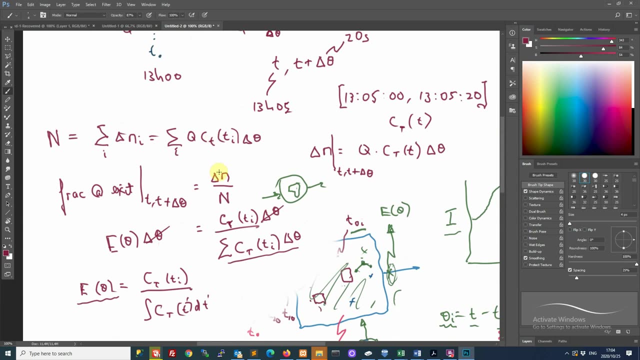 we want to estimate e of theta for any reactor. and if you think of it, we made no prescription on the nature of the mixing here. we didn't say that it had to be perfectly mixed for any of this to hold. but if you go back and think about, 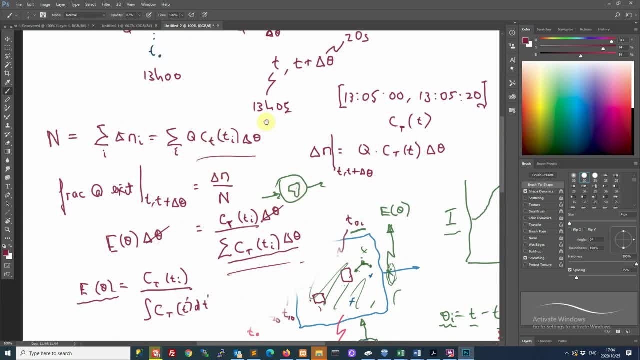 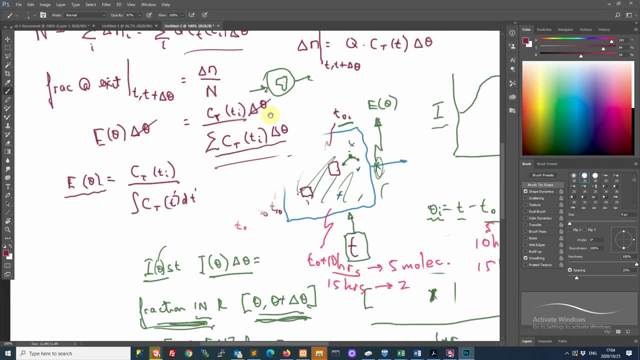 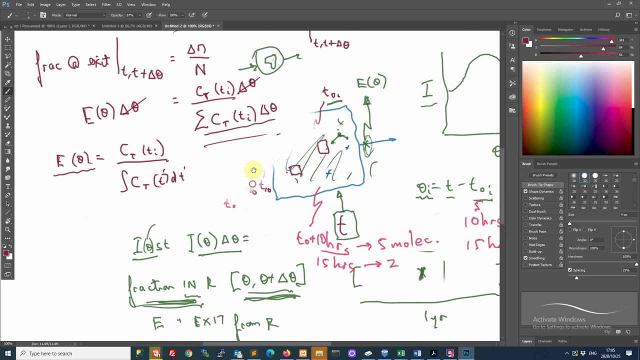 all these steps here. these are all simple definitions. we didn't need CSTR or PFR or batch reactor here. all we did was apply some basic Q times, C and and so on, with no assumptions behind those, and so this is generally true. right, this will work, no matter what type of mixing we have in. 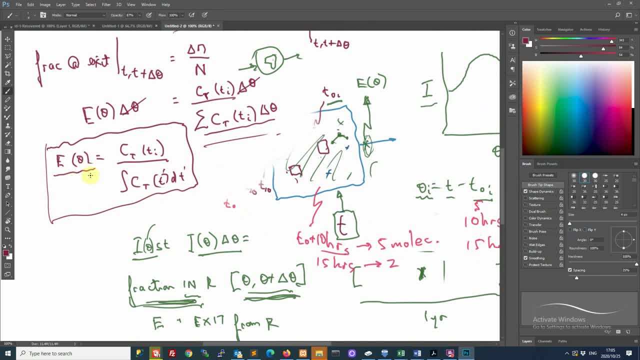 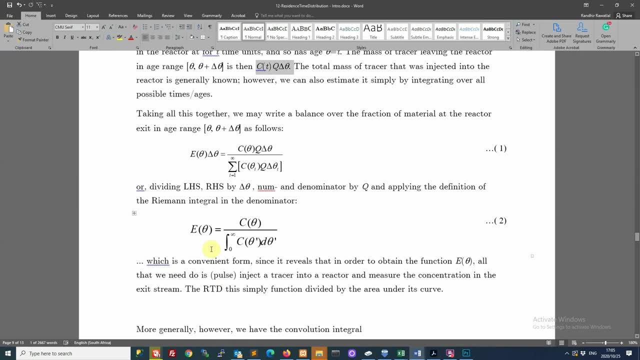 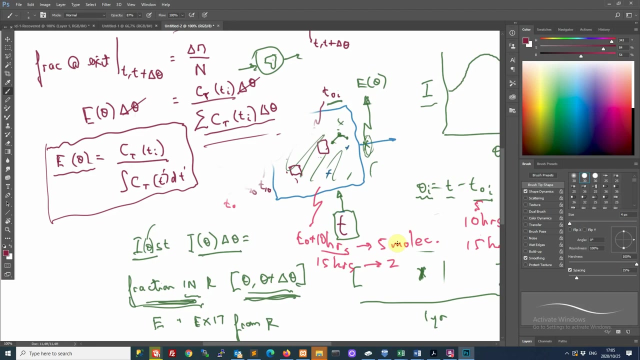 the reactor. so this is how we can estimate the exit age distribution from the reactor. so that's an intensely practical thing that we can do. we can, we can get the exit age distribution in the simple way. now, this was not exactly what we were talking about, right, when we were talking about this reactor. we were talking about 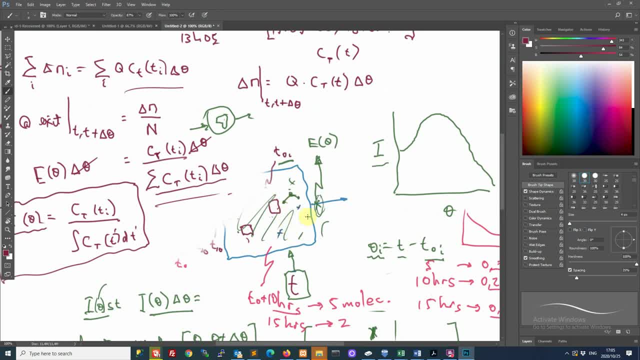 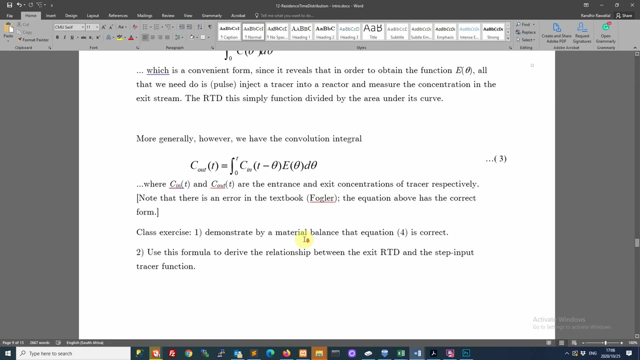 what proportion was in the reactor rather than at the exit point. so the other missing piece is the relationship between e of theta and I of theta, the internal age distribution. so we have now a nice way to estimate the exit age distribution. can we now figure out what the internal age distribution was? so to? 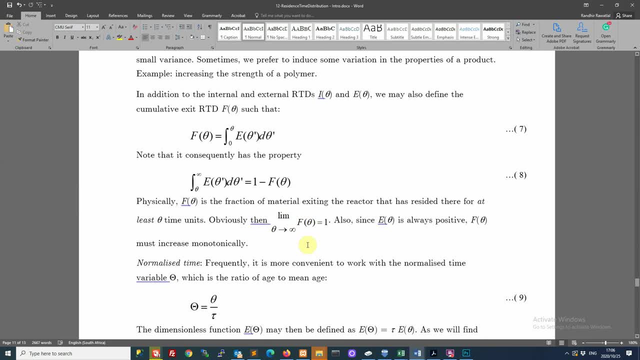 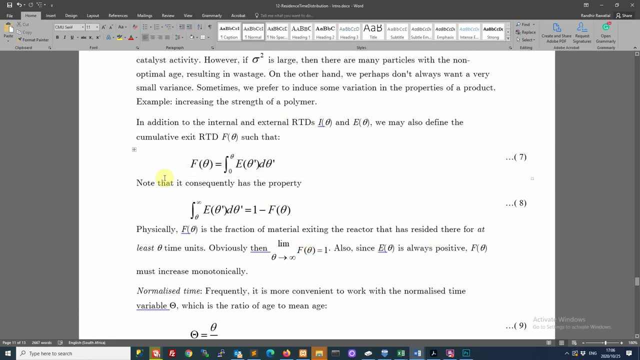 do that. I'm just being here. the first thing we are going to do is introduce this new definition: f of theta is the integral from naught to theta, e of theta. so remember, e of theta is the exit age distribution. so if we go and integrate from naught to theta, this is going to be the fraction of fluid elements that exit. 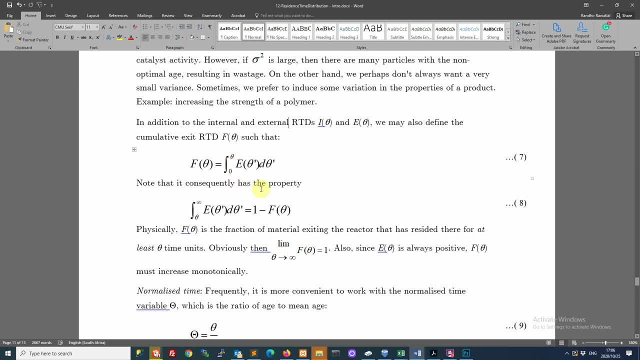 after age theta. so that's the fraction of fluid elements that spend at most theta in the reactor or having exited the reactor. so this is the fraction of. So this is the fraction of fluid elements up to a certain age that we observe at the exit right. 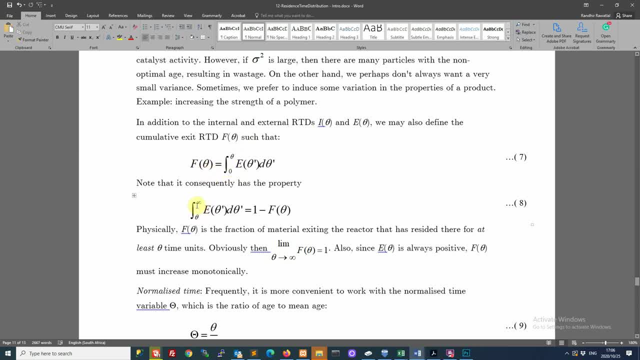 Now, the maximum possible age is infinity, right, Your lowest possible age is zero. You can't have a negative age. But in a reactor we can imagine we are aging to an infinite period. We could have a reaction space where things have been sitting there forever. 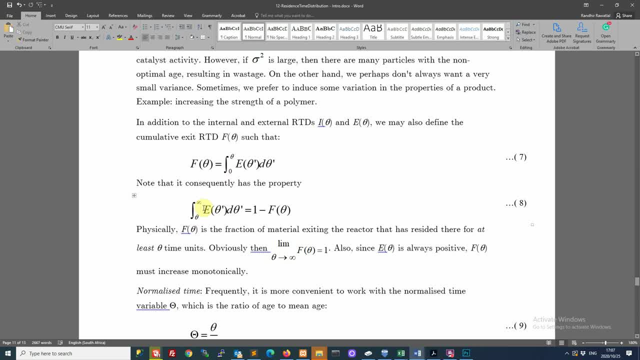 So it's not like a human population where we say, oh, the maximum age is something, And in fact we don't know that there is some maximum age. It's changing all the time. But anyway, in a chemical reactor we can certainly more generally say the maximum, there's no maximum. 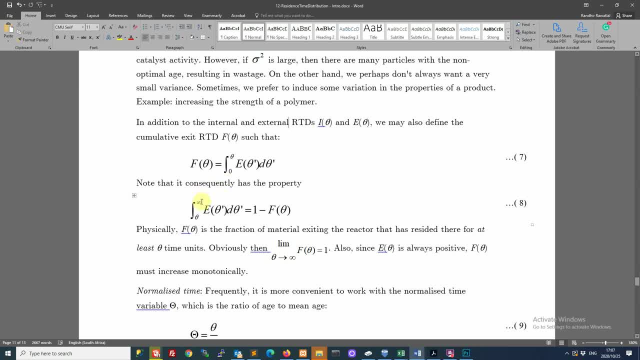 So we'll just go to infinity. So let's just leave it open and say: let's consider all ages onto infinity, And then we could say the fraction of fluid elements at the exit point of ages. at least theta can be represented this way, right? 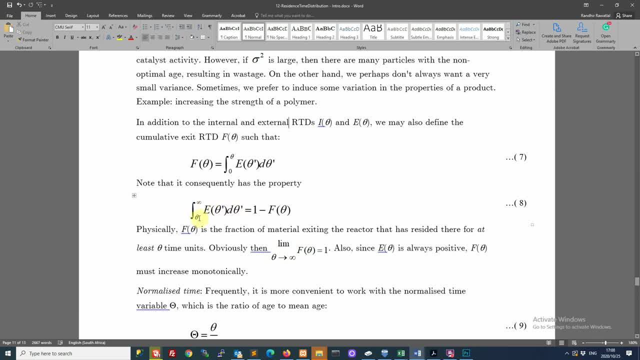 The fraction of ages, at least theta, So all fluid elements greater than or equal to the age of theta. that is obtained by integrating E of theta in this way, from theta to infinity, Right now. clearly, That is simply one minus this right. 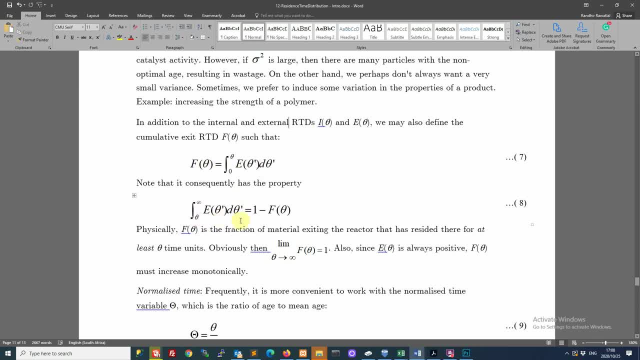 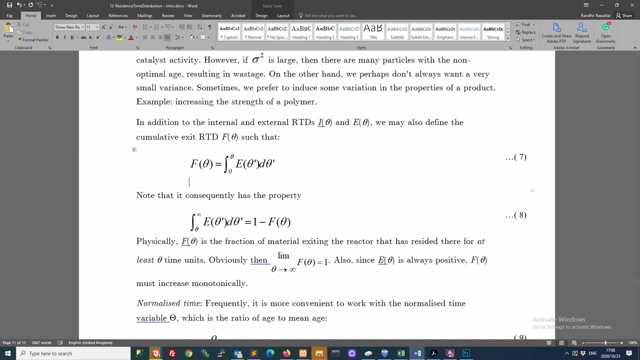 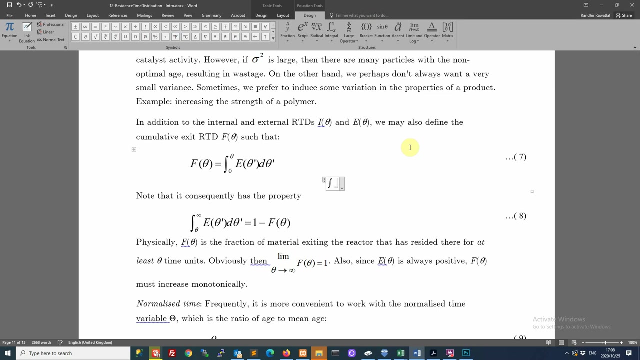 So the total fraction is of course one. If you add up all fluid elements, then the total fraction is a one right, Just by definition of fractions. So the integral from: yeah, maybe let's write it like this, We can say: the integral from naught. 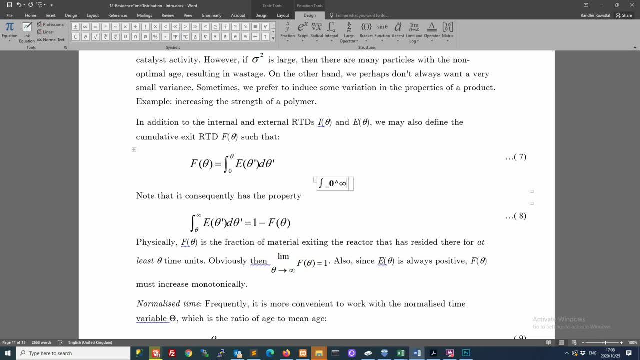 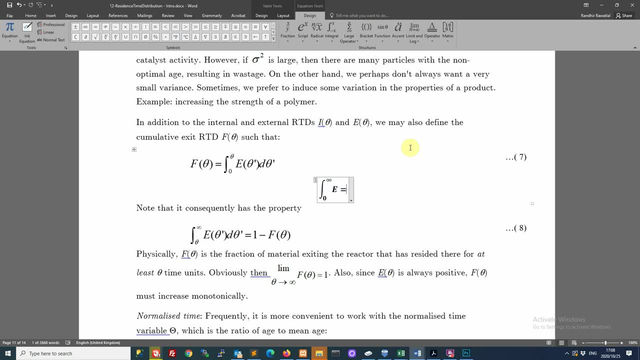 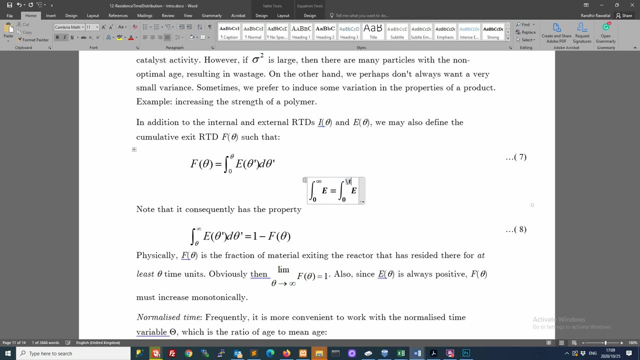 To infinity of E is equal to the integral from naught to theta plus the integral from theta to infinity Right. so we are going from naught to infinity, and we could simply interrupt this integration. We could. instead of going straight from naught to infinity, we can go naught to theta and then theta to infinity right. 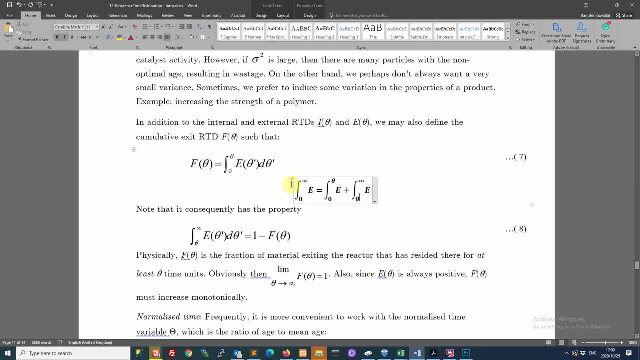 We know that's valid. Now, if we are integrating all possible fractions, right, that's another way to read this. right. All possible ages are naught to infinity. So if we add up all possible fractions, then that must simply be a one. 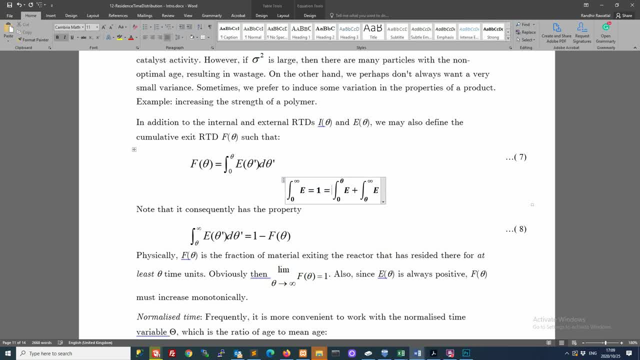 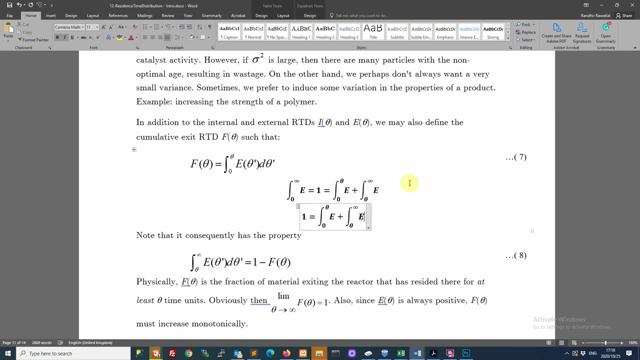 Right. so one equals that. So then we could say: naught to theta equals, and I'm just going to copy it like this: So naught to theta or naught to infinity, or theta to infinity is one minus naught Right, which is the same as one minus f of theta. 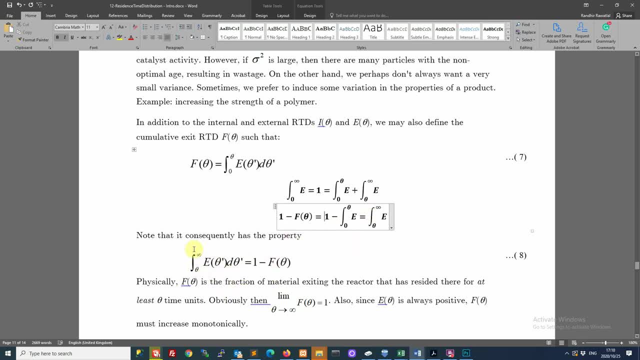 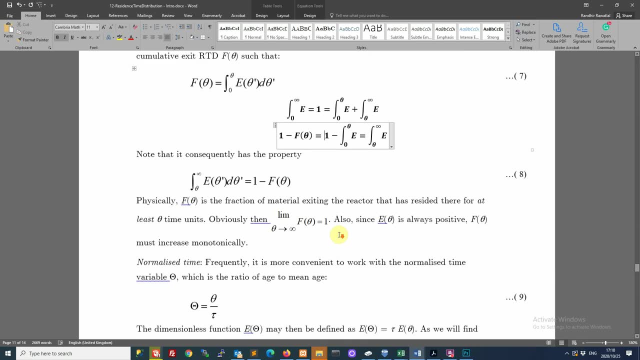 Right, so that's what that means. So if you want the fraction of fluid elements of age, at least theta, then that's what you have. So, anyway, that's all rather formal. Let's again think about a material balance around this. 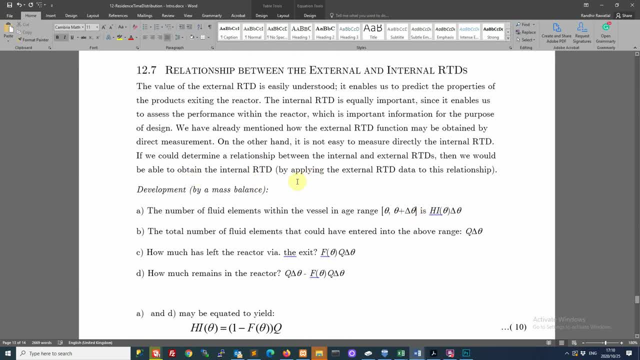 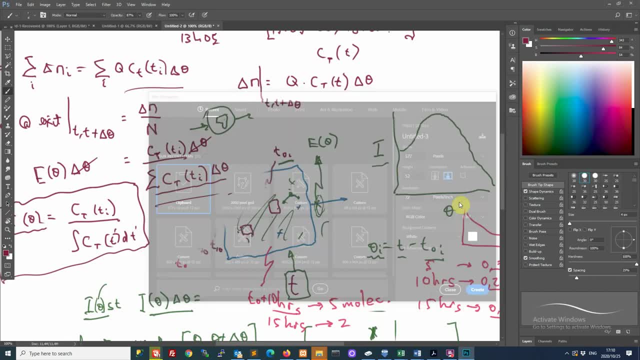 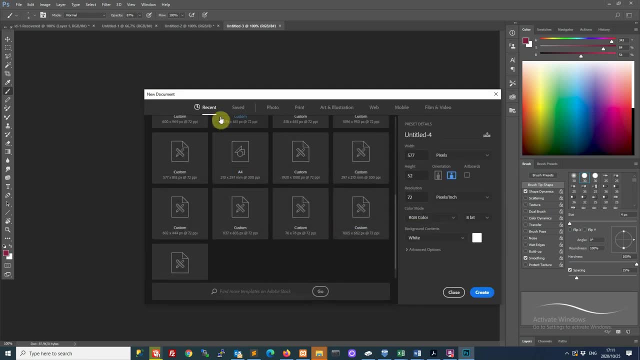 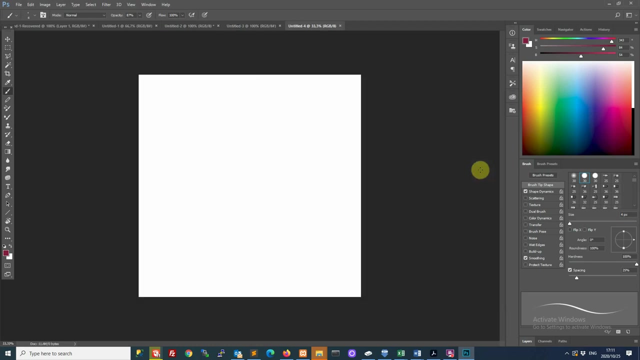 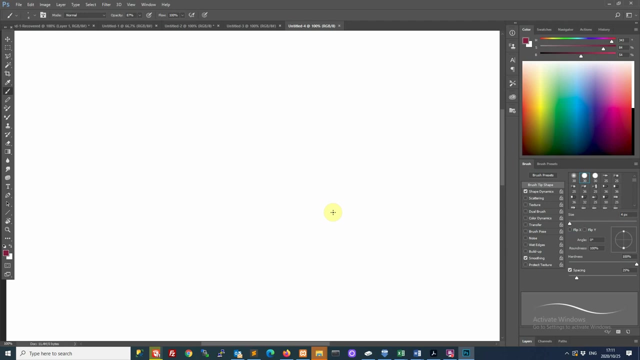 So, having established, So, having established that let's think about a fluid- well, fluid- element in some vessel. Let's just clean up here a bit. So let's think about a space where We've introduced our fluid elements into the reactor, but the system kept flowing. 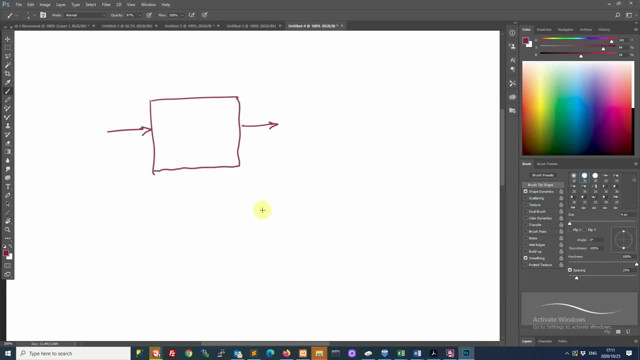 and we are now interested in some instant in time t We've fed everything in at time t naught, and so over time we have been observing that our fluid elements have been leaving. So we spiked everything in. So we spiked everything in at time t naught, and so over time we have been observing that our fluid elements have been leaving. 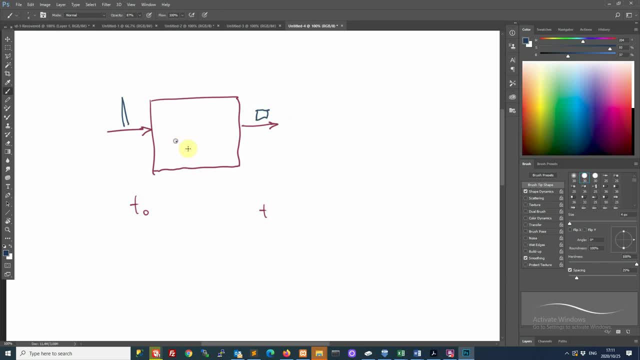 So we can see that this spiked everything in at time t naught, Then they distribute it in here And then, between t naught and t, our fluid elements have been escaping the system. So we would like to have an accounting of the amount of tracer left over in that reactor. 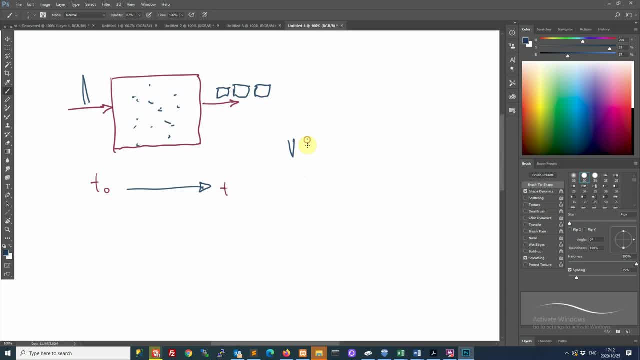 We can talk about the volume of the space and I of theta. so we know the fraction left over in the reactor is I of theta, Delta theta, right by definition of that distribution function. this is the fraction of fluid elements in age, theta to theta plus Delta theta, in the reactor. 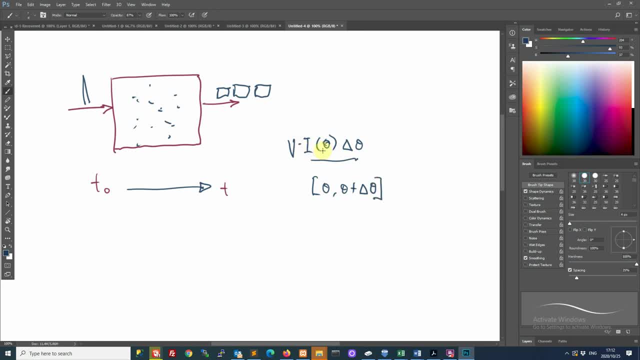 right. so if we multiply that by V, then that's the total volume of fluid elements of that age, of that age range, in the reactor. that must equal the number of fluid elements, that of this age range, that entered in the first place. and if you think of it, the amount that entered in the first place was Q. 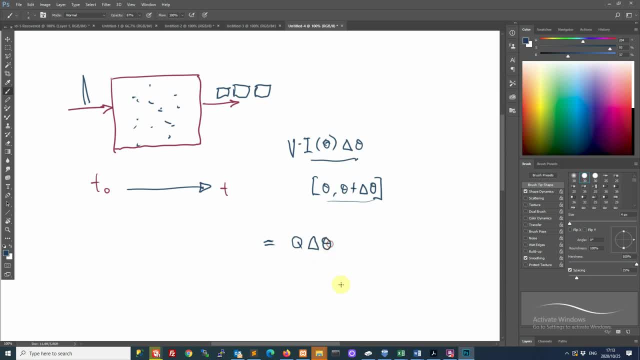 and the time range is Delta theta. so, if you like, this is the total amount of fluid elements that that entered the reactor in the first place that could possibly be sitting in this age range. now, right, so this age range has a width of Delta theta, so there's a certain period of time that passed Delta. this thing looks. 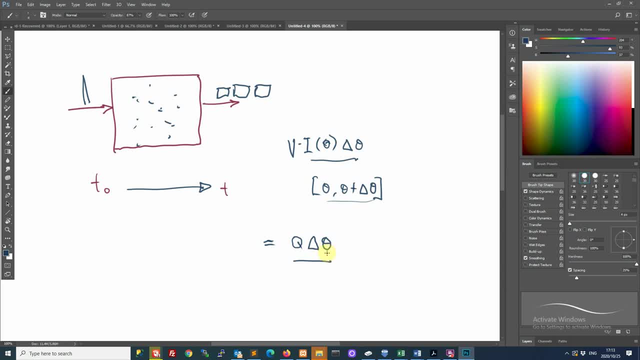 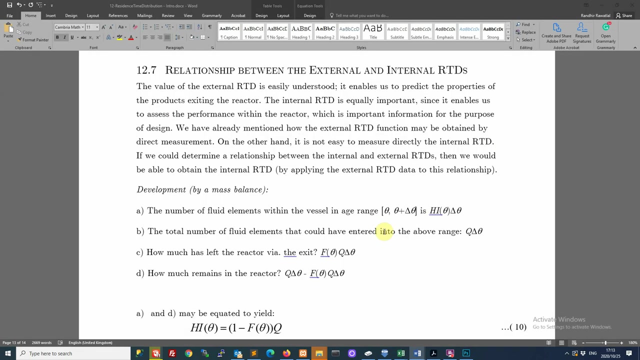 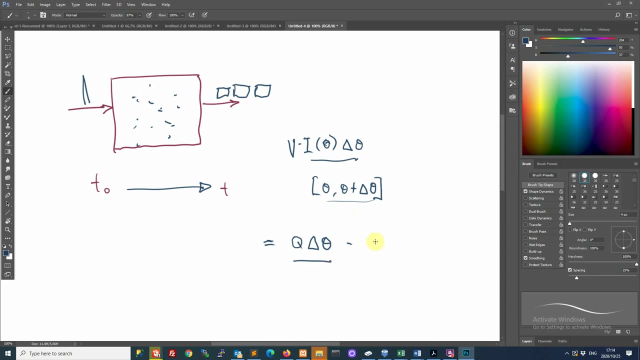 kind of like a face. so anyway, a Delta, theta, that that's. that's what's passed. and now, this is the amount that entered in the first place, and then the amount of this that exited. that must be the amount that's at the exit point, that that's going to be the contribution of all ages earlier than. 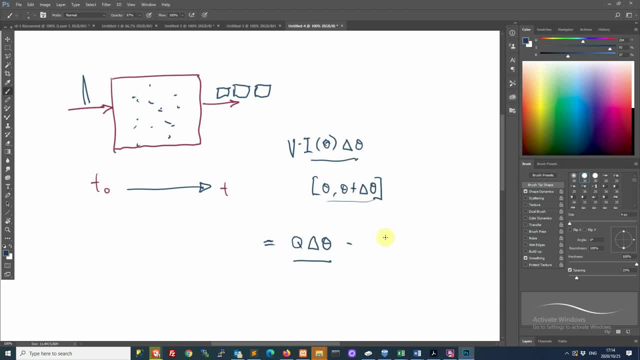 current time, that then age of interest theta. so the integral of all those ages so naught, 2 theta. so that's going to be the fraction that was exiting during that time. so here I'm going to write this as, in terms of flow, e of theta. 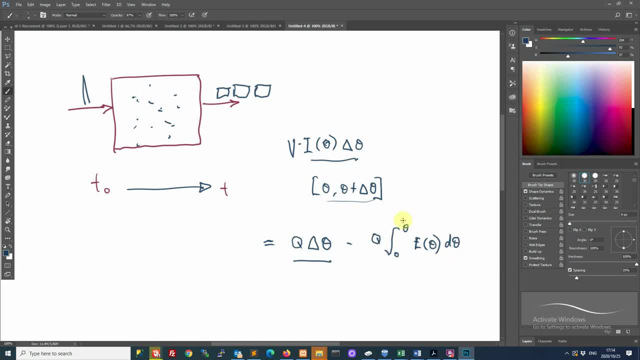 if you integrate this, this is the fraction that left the reactor. so up to age theta. remember: now we are only interested in age theta here and only between theta and theta plus delta theta. we only want to know how much is left over in the reactor of that age range. 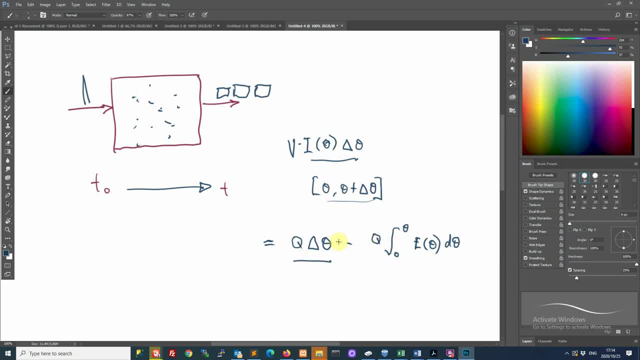 so we are trying to estimate how much could have been there. so if nothing exited at all, then that's possibly how much would be in the reactor. however, we know that we did lose some fluid exit elements due to flow, but we've got e of theta and we know how to measure that. 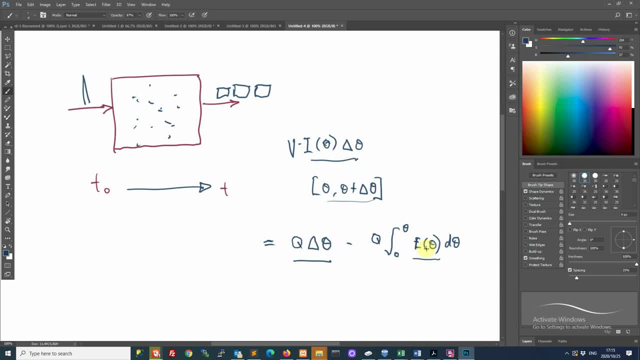 we established the trace experiment and that can give us e of theta. so we could simply integrate this and that would tell us the fraction of fluid elements that exited the reactor, so that fraction times that flow, that tells us how much has exited the reactor. and then, of course, we have to multiply this by delta theta, because that's 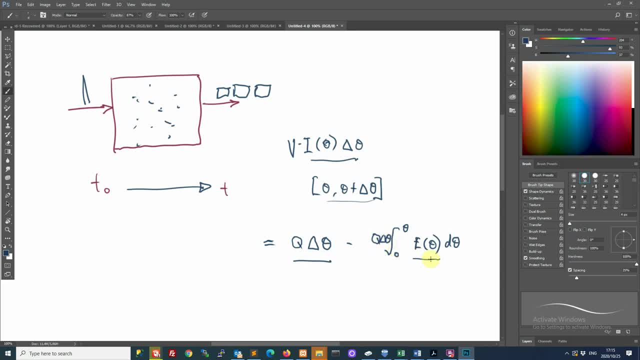 the fraction, but we need to know how much has exited the reactor. multiply by the number of fluid elements that exited also. so then, if you rewrite this as sorry, Q, Q, Delta theta times 1 minus integral naught to theta E of theta, that's equal to ve I of theta, Delta theta, and you can see the. 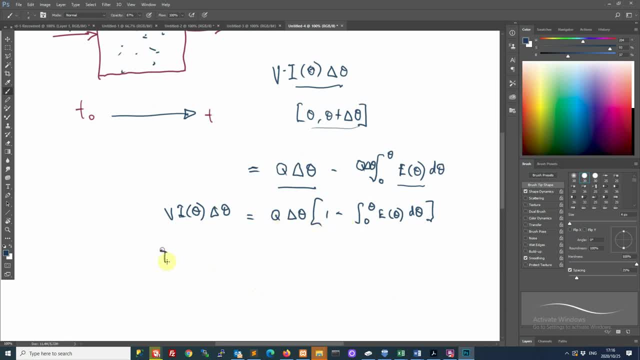 relationship- now you can see, I of theta is. then simply you can divide v, Delta, theta, so Q over V is 1 over tau, so this is 1 over delta. so we can write it as theta, delta, theta, because that's a R and the over tau, and then the delta thetas can cancel, leaving us with simply 1, 1 minus the integral. 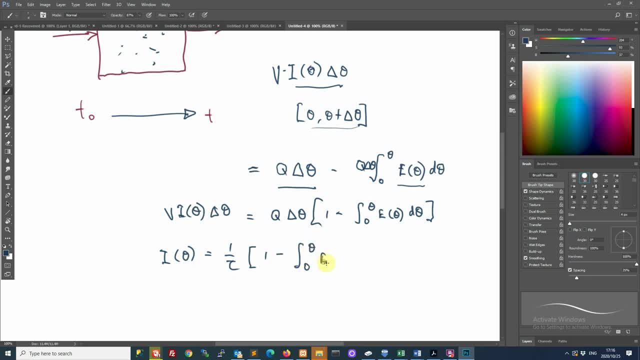 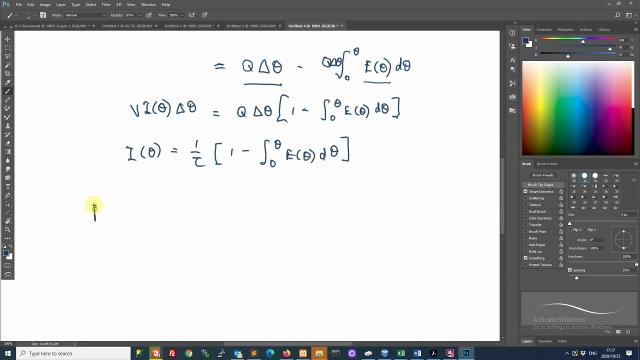 0 to theta. e of theta, And that's the other half of it, right? We know how to get e of theta quite easily. e of theta is simply the concentration of tracer, the function that you get divided by the area under that function, And in fact I should say here theta instead. 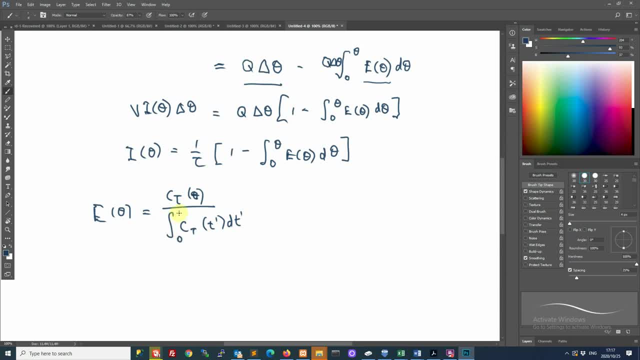 of t, So you just integrate under this function, So that gives you e of theta. So e of theta is some function, So it's something, whatever it is, And then we can stick that same function in here and we can get i of theta, So that's.